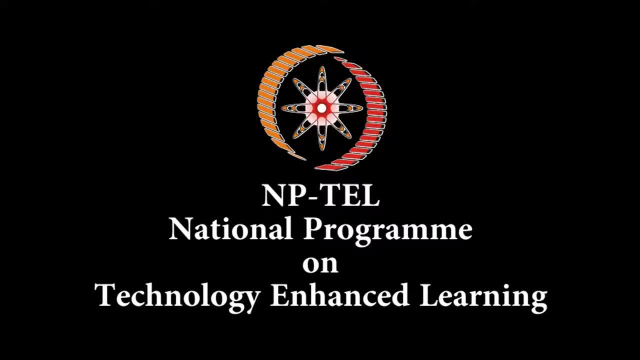 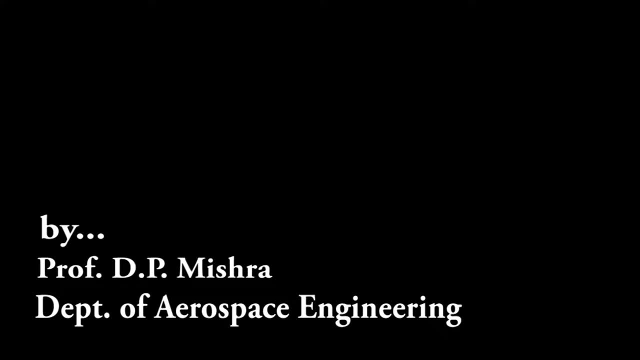 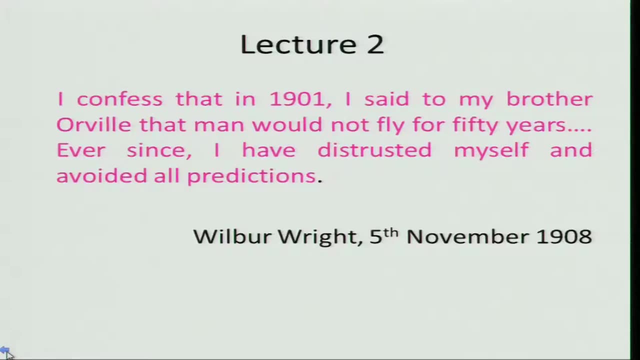 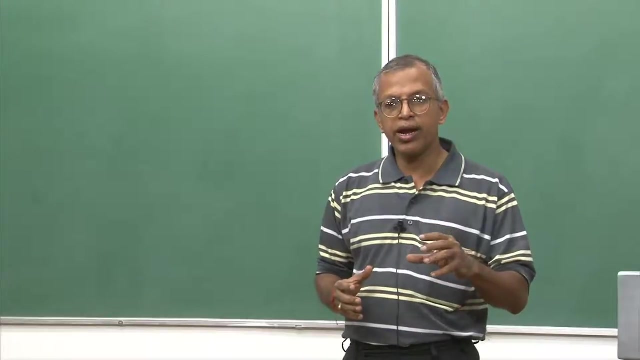 Let us start this lecture 2.. Before getting into this lecture 2, what we will do, We will try to recall what we learned in the last lecture In this course. what we will be looking at? Aerothermodynamics of the propulsion. That means we will be looking at how to convert. 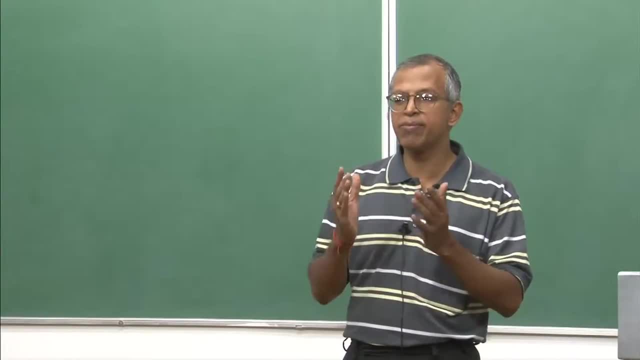 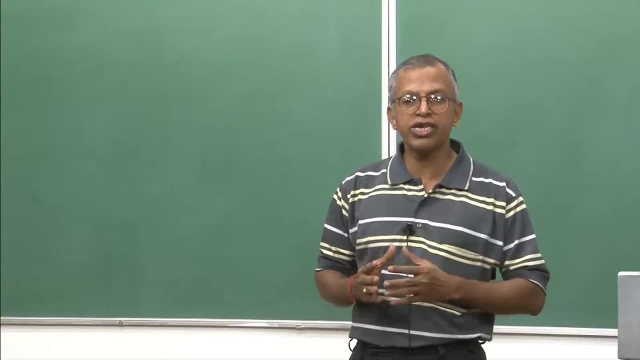 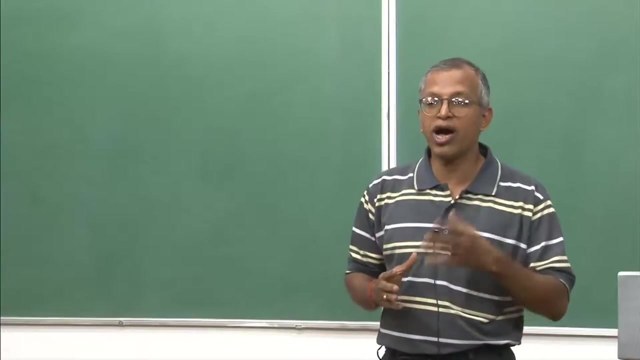 this energy into the thrust power. So that is the basic idea in this course. Subsequently, in the last lecture we discussed about how the propulsion evolved in terms of history. I ask a question: why really we want to have propulsion? 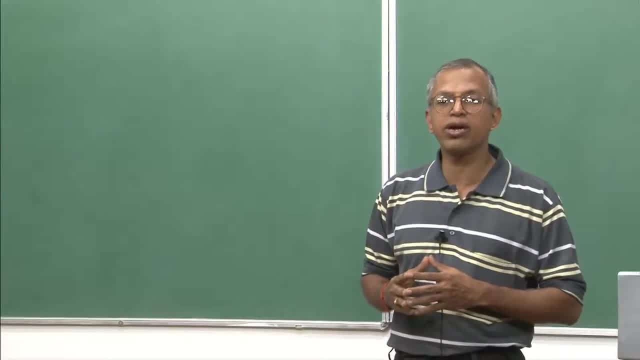 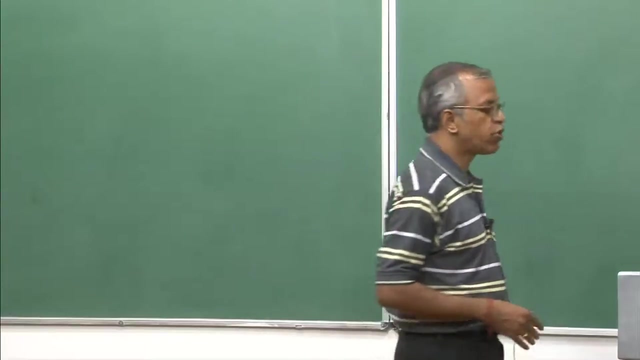 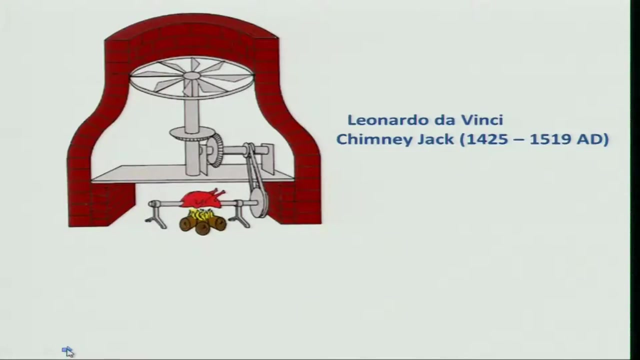 Look at history. It is important because we need to learn the way they have developed the processes such that it will be useful for today to apply it, such that our future will be better. We will look at those things, some portion. Let us look at Leonardo da Vinci. 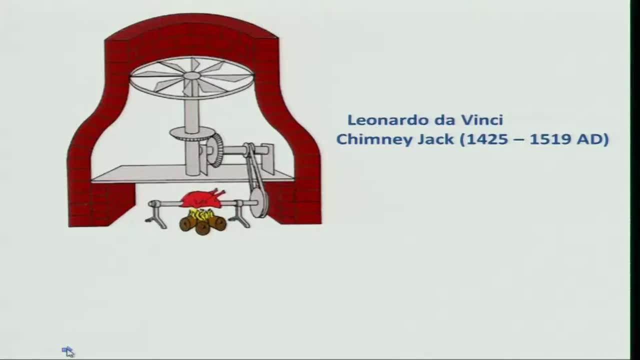 really, who devised this chimney giant? If you look at, these are the pictures which I have shown here. This is a turbine which will be rotating. This turbine is connected to the shaft through a gear trains and also a lever pulley which is joined with this roasting pit. How does it work? If you look. 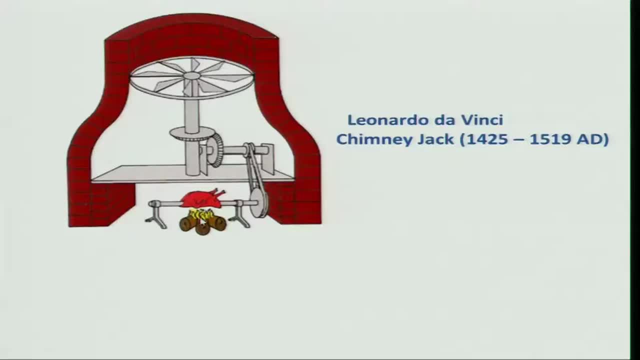 at it. Basically, it burns this wood, which is being burned to provide the heat to this roasting speed. What is that? It is basically a place which is being to be cooked. This pit will be rotated. Now, this burning of this, what you call this flesh or a meat, the burning 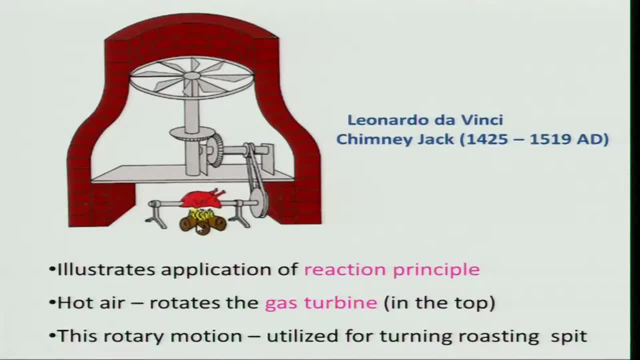 of this wood will be producing the gas. This gas will be producing the gas. This gas will be passing through this turbine which will rotate it. If you look at this, this is the first concept which was being sketched by a Leonardo da Vinci who is not involved in. 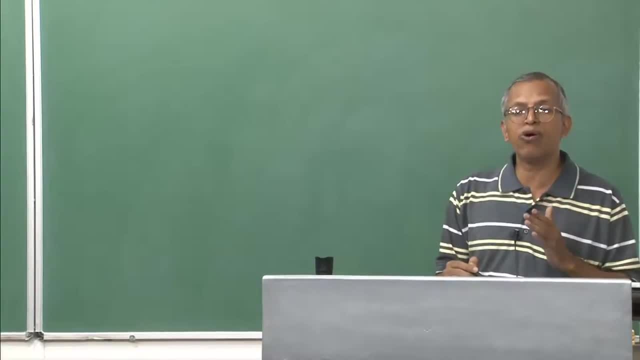 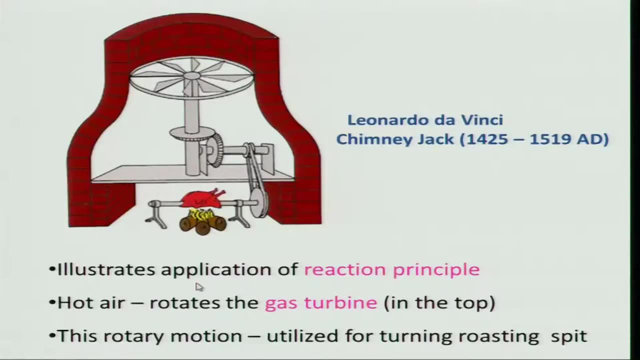 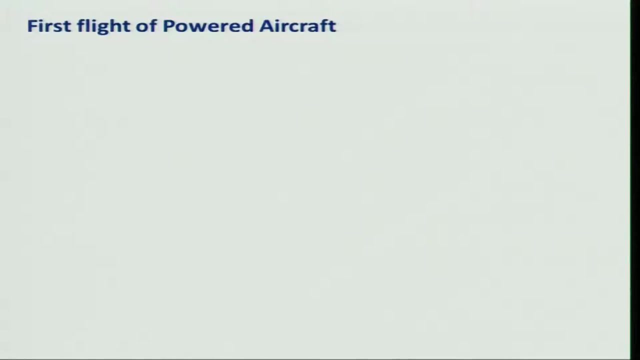 the science activities. However, he was known as a greatest artist. He illustrated this application of reaction principle. So now we will be moving into the first flight of the aircraft and which had made a epoch in the history of aircraft propulsion. So if 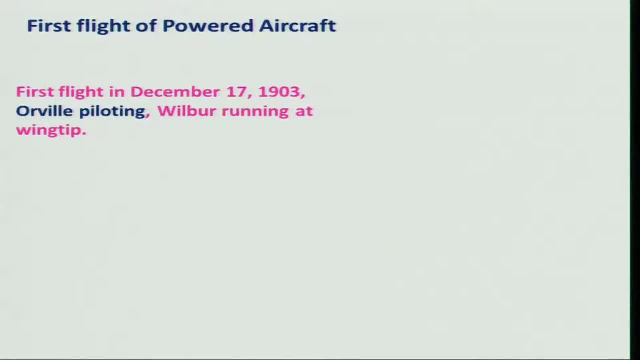 you look at, it was basically done by this Wright brothers in December 17903,. he flew the first flight And if you look at, his flight is pictures I have shown here that this is the flight which is here and it is having a propeller which is not visible in this figure. 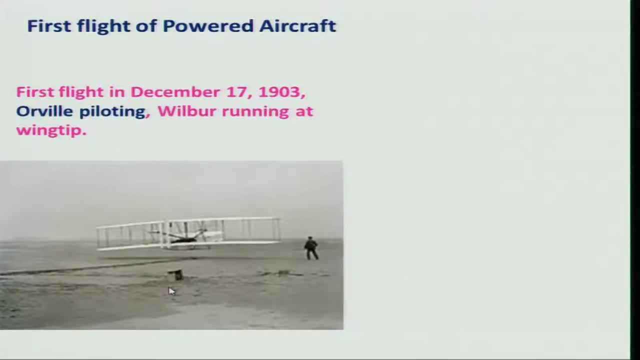 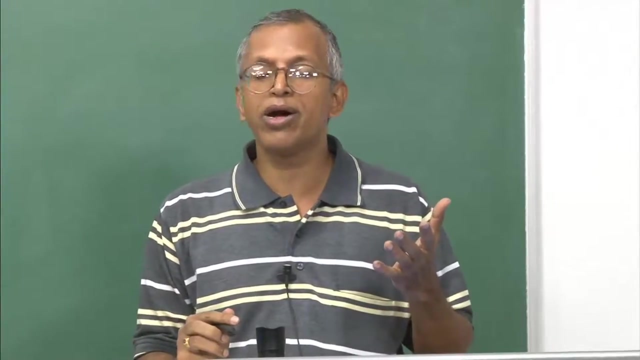 and or while pilot link this flight, whereas Wilbur is standing here at the wing tip to look at how it is flying. Do you know how? what is the? The duration of time it flew? it was only for 100, 12 seconds, and it could cover 120 feet. 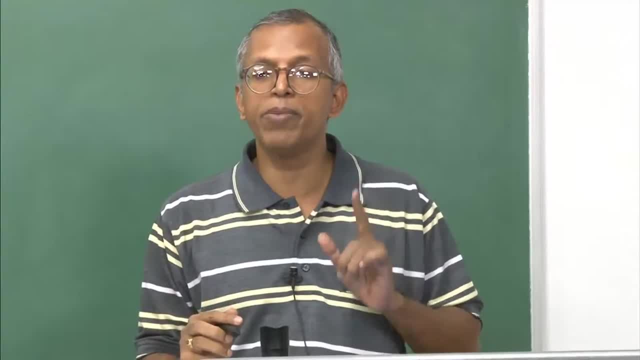 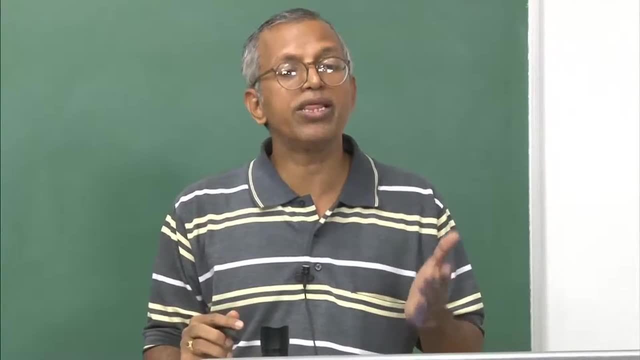 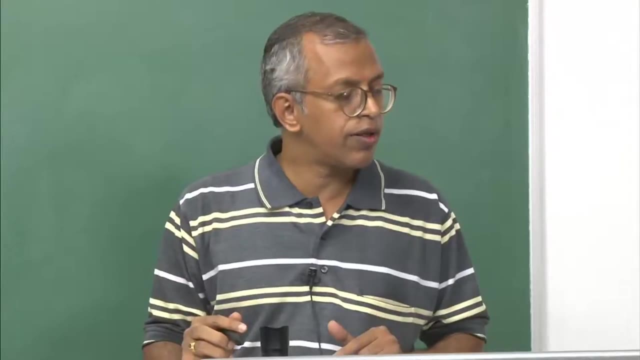 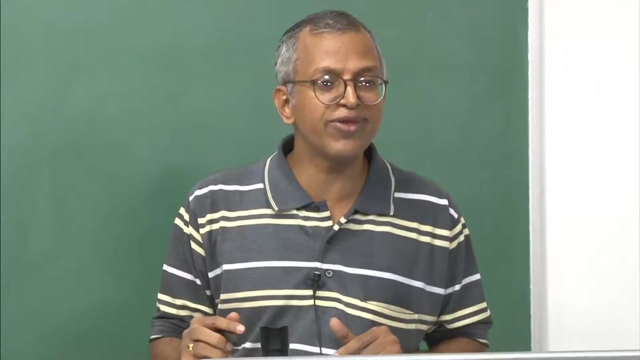 kind of things, and after that it was no, but however, it made an history. But if you look at these two brothers who worked relentlessly with lot of failures- If you remember that first slide, I showed you that with frustration, that or while told to his brother that man cannot fly for next 50 years- but they proved that, yes, it is possible. 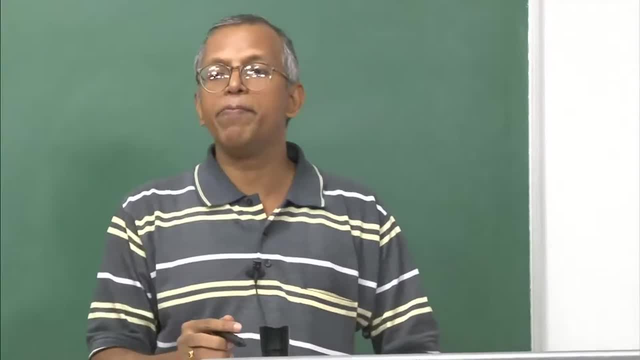 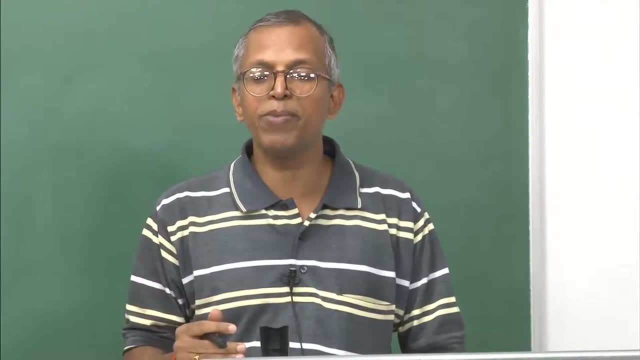 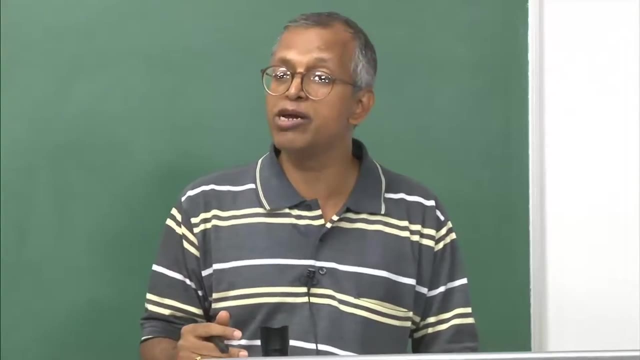 So therefore, engineering, per say it is being done with a lot of failures, but if you look at today's mind, set that first failure make us to be depressed So that we will leave that and go somewhere else. engineering cannot be done that way, I must tell you. and those 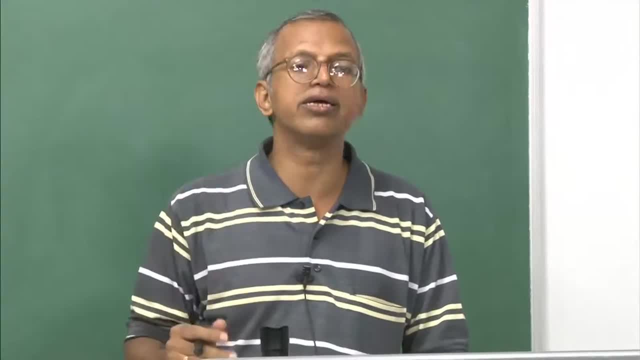 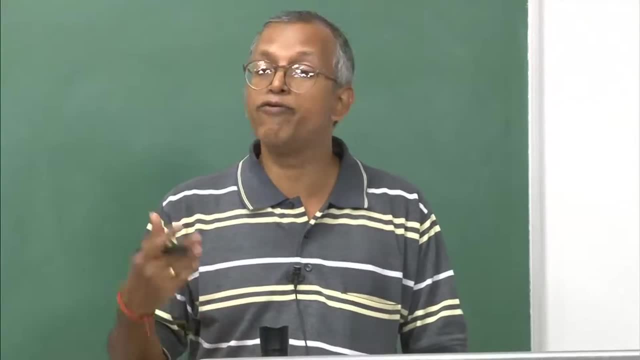 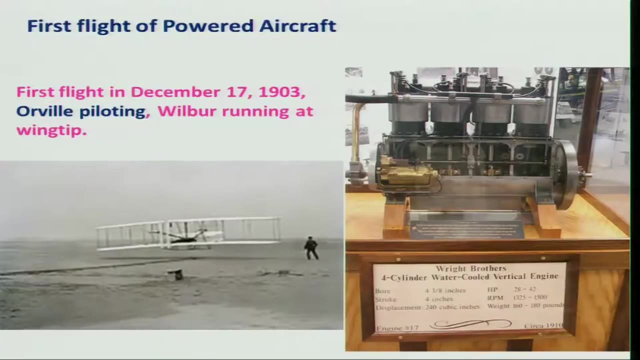 people who have developed the engines or any other Kind of success they got. they got all those thing with persistent report and with a lot of failures. So therefore, failure is the pillar of the success, as being told, and they used a what you call a in line engines and which will be discussing about it, and it is. 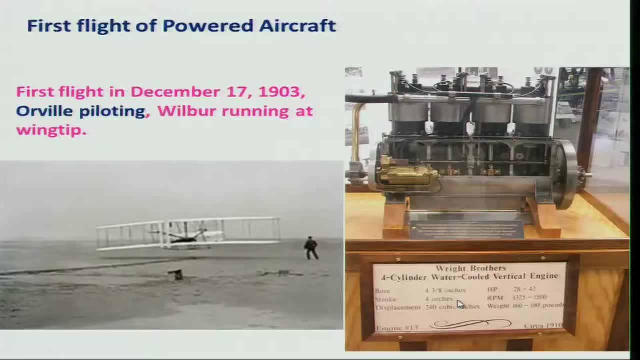 basically a four cylinder water cool vertical engines and the figure is shown and it is being done by design by a Charlie. If you look at, it is not a single man job to have an aircraft or a any engineering product. it is the group work which is very essential. and whenever you are working in a group and 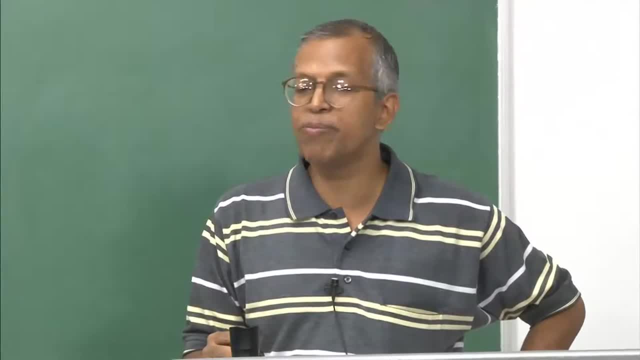 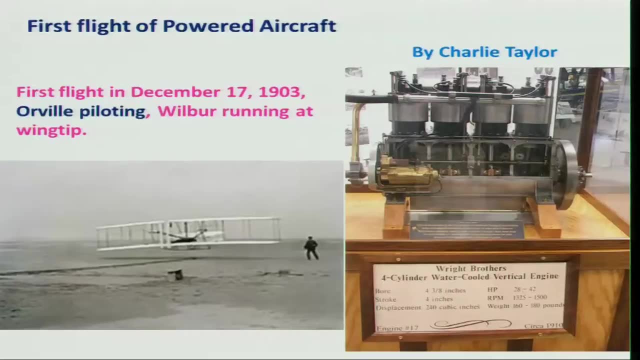 you will have to adjust with the people and which is lacking in the present modern India, that we became more secluded and single minded. that would not fetch us engineering. So therefore, this is the quite good lesson we should learn from this development, And it was really created a history. now this, after this development: the most of the aircraft 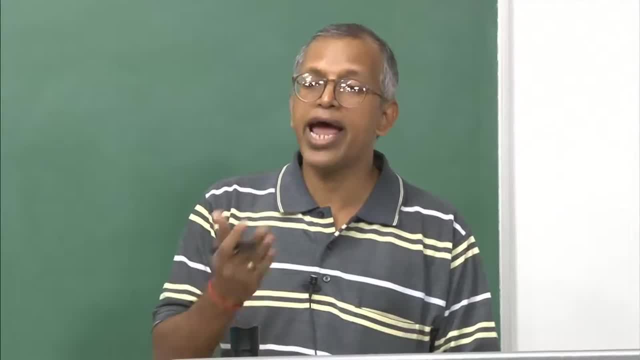 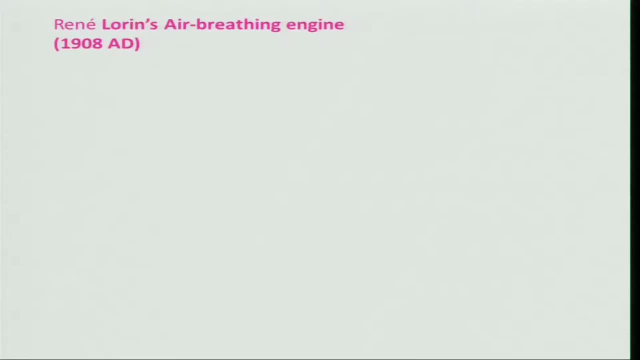 is being propelled by the propeller and with the help of power plant known as I C engine. And, of course, the air breathing engine concept was given by a genius- I call it Rene Laurin- and who gave a concept taking from the piston engine. 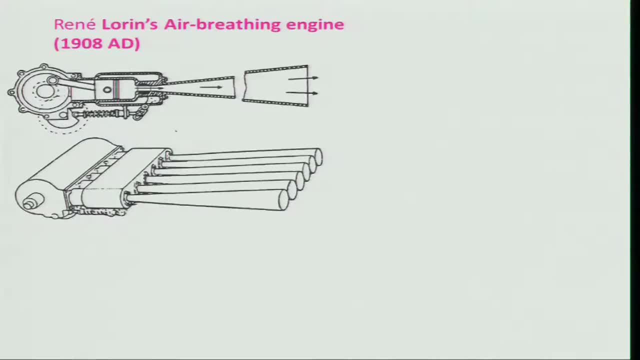 I will show you a figure here. and in this case, this engine is basically connected with a, with a nozzle which is- you can call it as a conversion diverter nozzle, and this is the cross sectional view and this is the number of nozzles which are connected to a in line. 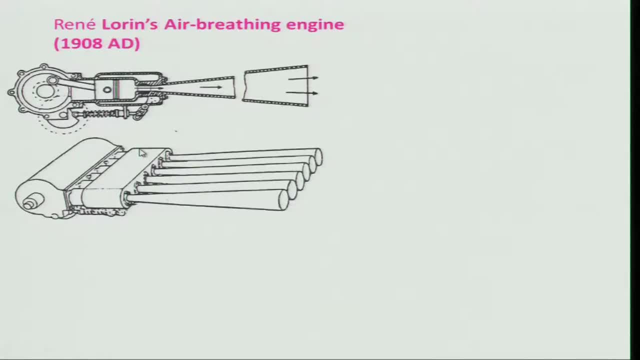 engine. If you look at this is basically in line engine and he gave this concept of piston engine converting piston engine air breathing. that means is basically concept of jet engine you can call And of course the piston engine is an air breathing engine because it takes the air and use what you 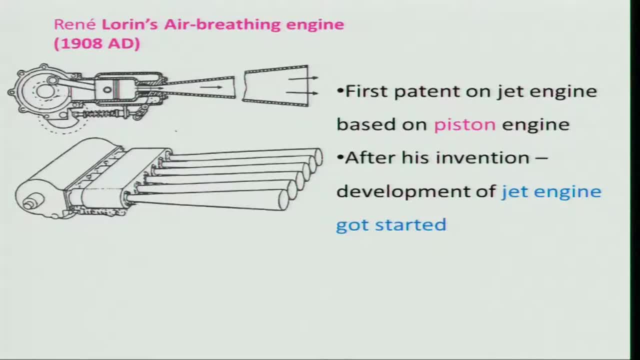 call for burning the fuel, So it is an air breathing engine. However, the jet engine concept was given by Len Lauren in 1908 and he gave another beautiful concept in 1913 AD and which is the ram jet engine that we use today for the missile applications And 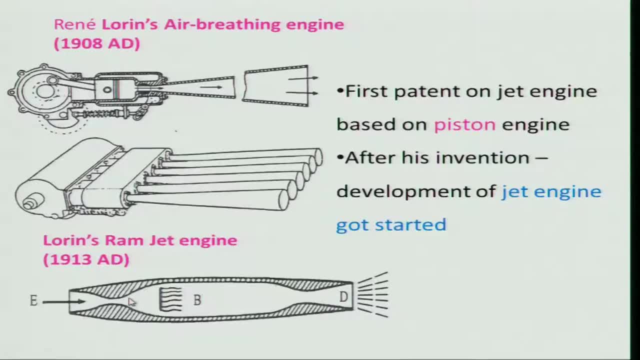 if you look at, this is having a what you call a diffuser or air intake, which of course work in a supersonic flight, and it is having a combustion chamber and a nozzle. So if you look at it is not having any rotary components or any complicated components. 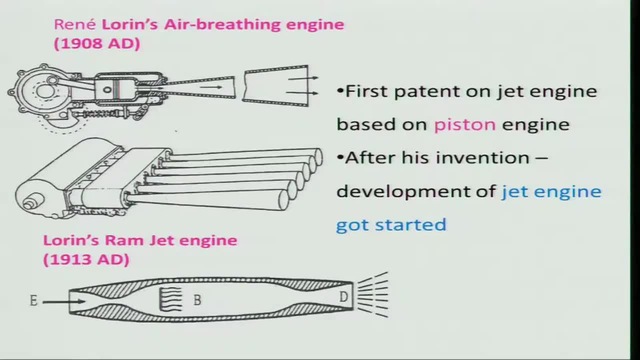 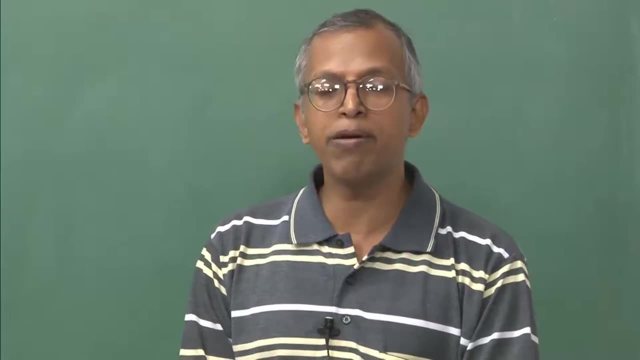 It is a mere duct which you give the thrust. So, if you look at, these are the concept which was given by Lauren, and he is a known to be a great innovators. So what is important for engineering is innovation, and person should be creative in nature But unfortunately, 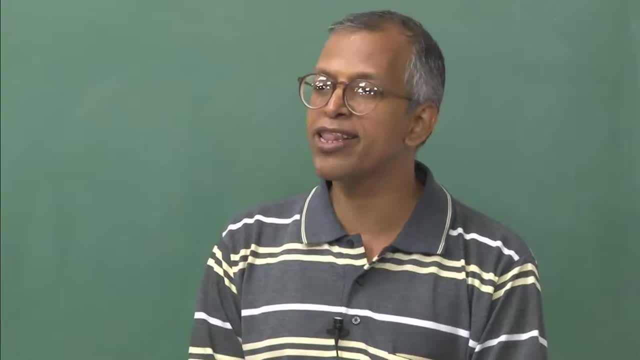 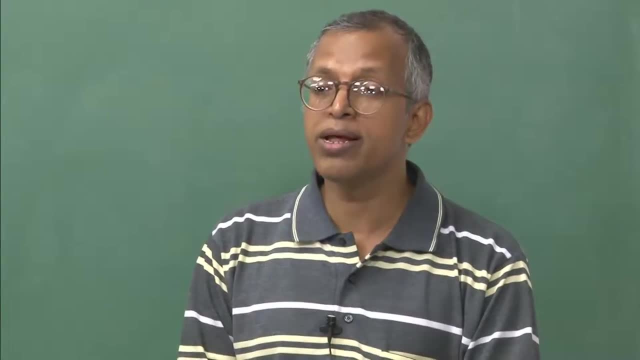 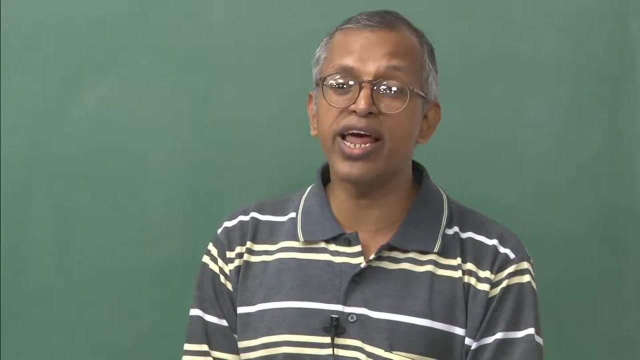 today we are not that creative because of fact that we are working quite hard and all always busy in something or other. but the man innate nature is creative. I always say that man is a creative creature by nature. Unfortunately, modern education system and the societal society is not allowing us to go back to our own nature and develop and 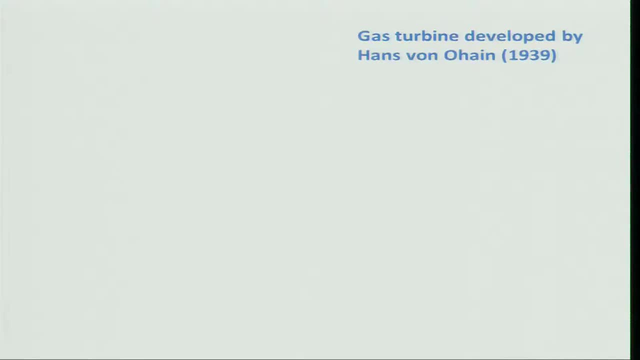 work for others. So, coming back to that, I will tell you that this after that, subsequently, 1930 AD, In 1939, there is a person, German, Hans von Ohen, who developed the gas turbine engine, but most of you will be telling me that it is the Whittle, sir Whittle, who developed the. 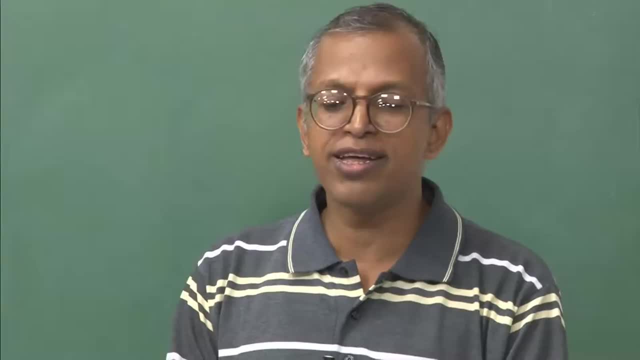 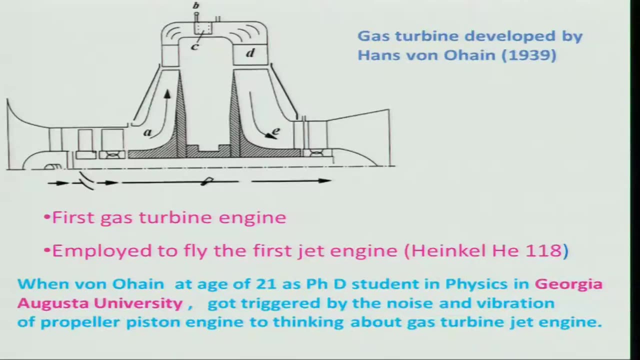 gas turbine engine. but it is actually the von Ohen who, when he was a student in a PhD student in the Georgia Augusta University at the age of 21. And enrolled as a PhD program in physics. he was never a engineer and he got annoyed. 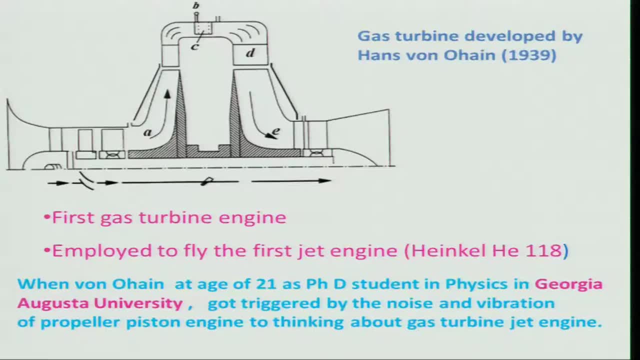 by the noise and vibration created by the propeller piston engine in his lab. And then he thought about why not have a engine which will be smooth enough and it would not cause any noise or vibration At the same time, it will be smooth enough and it will not cause 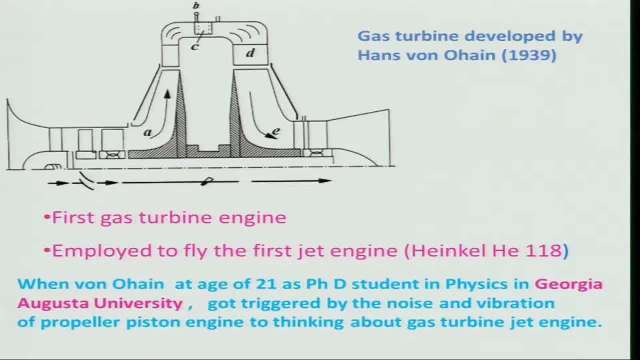 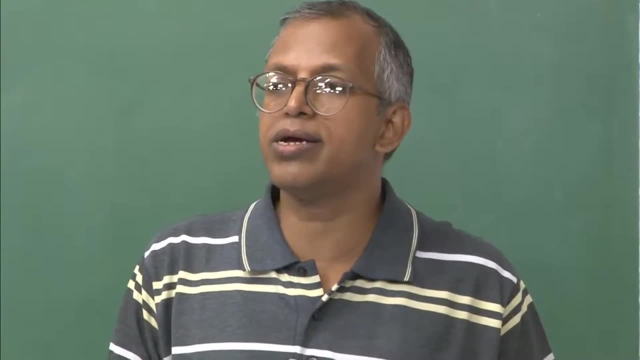 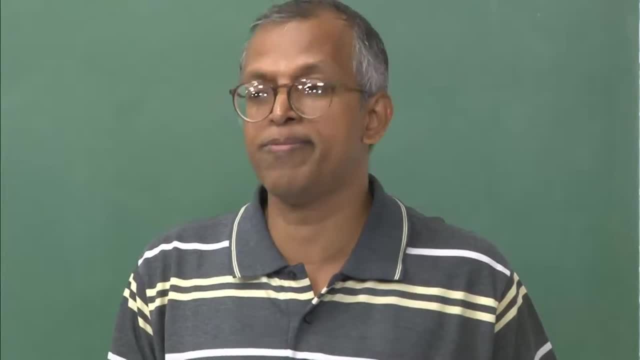 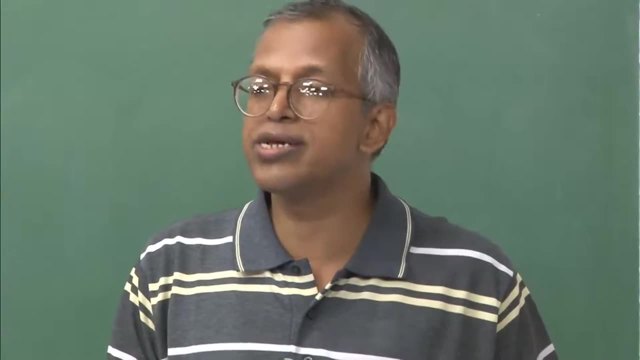 for quite some time, till you finished his PhD. He did not run away from the P S D program. he finished his Ph D and then he requested his professor Paul to write a recommendation to another person whose name was Anthony SS. Thank you, Professor. you may go ahead. 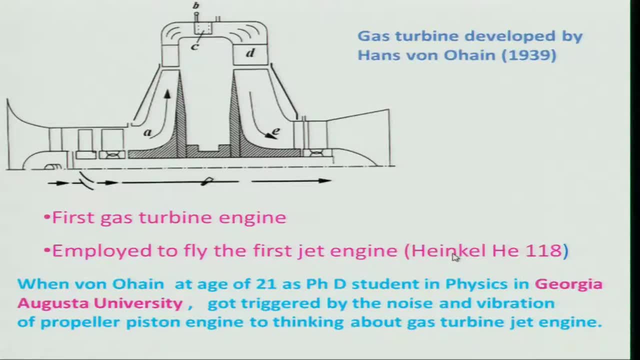 Thank you, Professor, you, you may go ahead. Thank you, professor, you may go ahead. I reallyEach one proposal I will give you. you, we will build a gas turbine, understand, whose name is Henkel. Henkel is a basically proprietor of a aircraft engines. and then 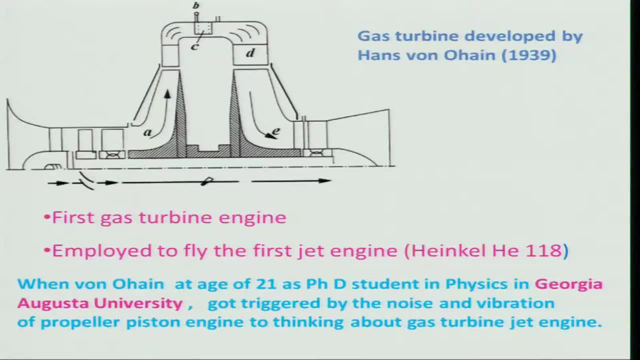 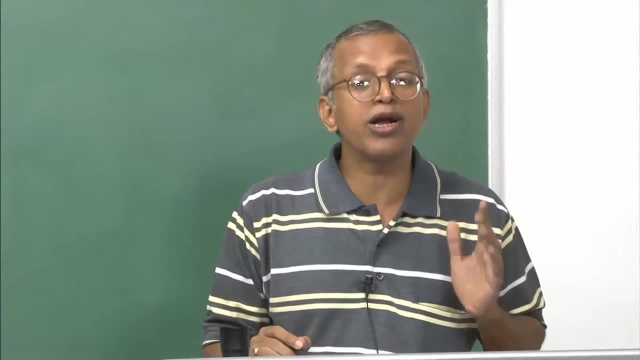 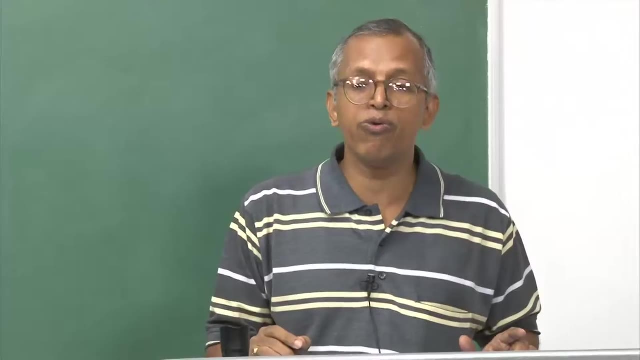 he introduced Henkel was very encouraging, but at the same time he is a business man. he was a business man and he was reluctant to take of this thing He convince as a young person and worked hard with a lot of constraint and came up with a engine which cross section. 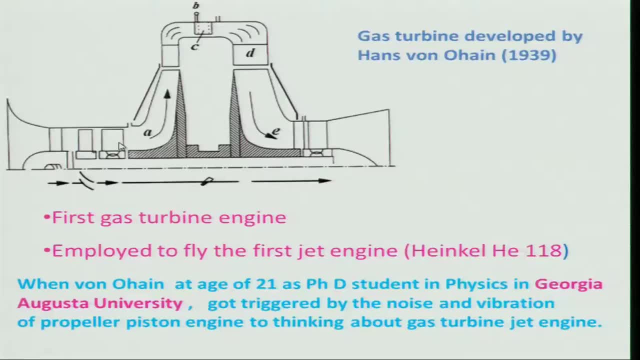 I have shown here. It is having a air intake and then there is a radial compressor, there is a combustion chamber and it is having a turbine. and he flew that in 1939 as a first aircraft to be flown by the gas turbine jet engine. 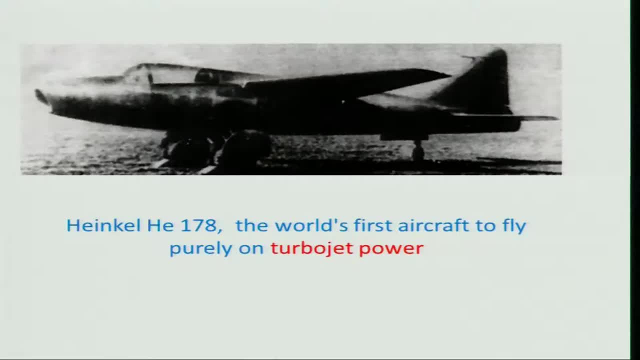 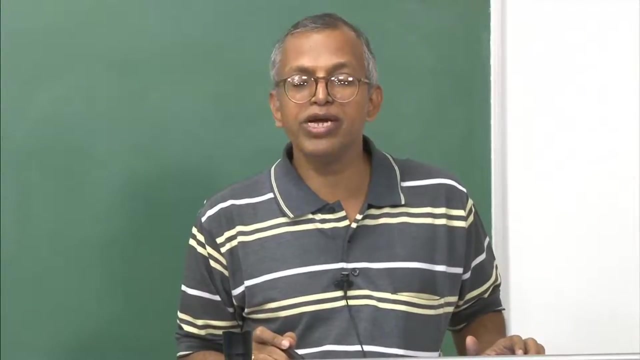 So, if you look at- and this is the first engine ever- engine was being flown by the turbo jet power in which hydrogen as a fuel is being used. Today, people are contemplating to use the hydrogen as a aviation fuel for aircraft because of stringent pollution or 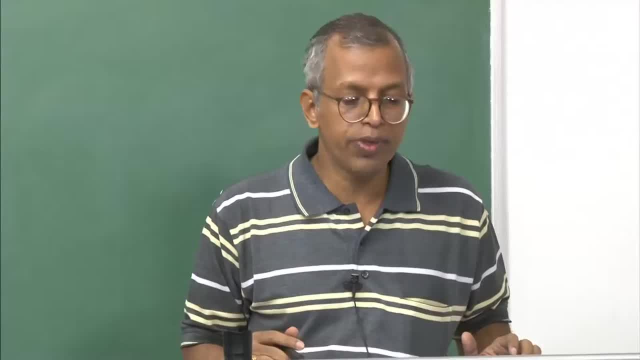 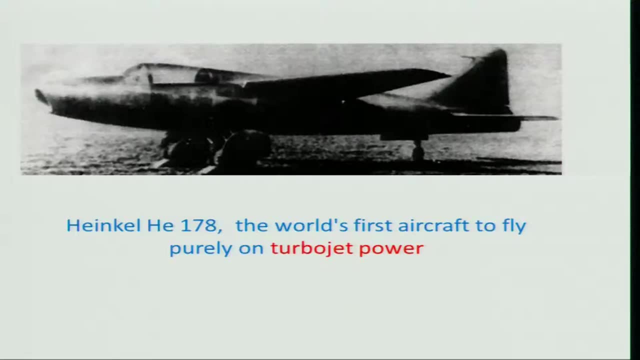 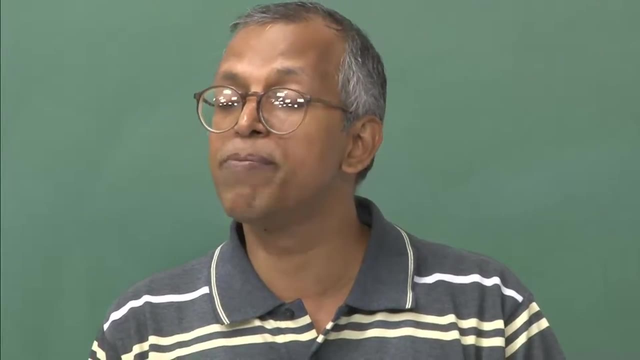 the problems being faced by across the globe. And he was the first person, but he was never consider as a inventor of gas turbine engine because of fact that the German lost the war in the second world war. So therefore he was, but fortunately, and I am also very delighted. 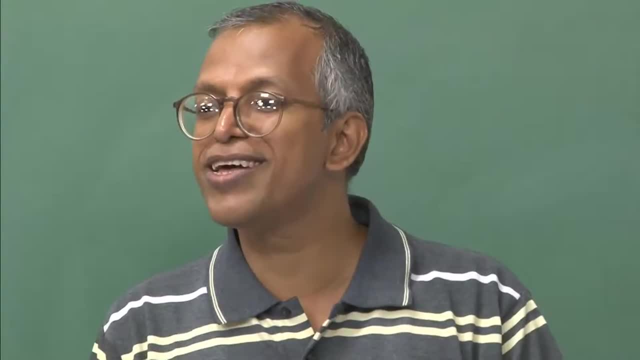 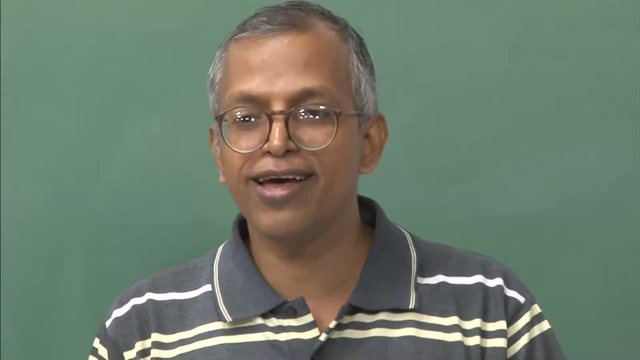 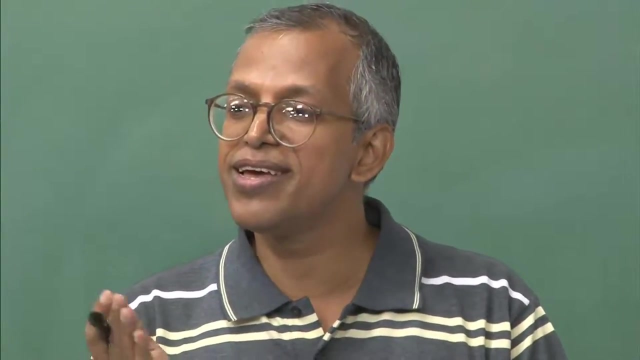 that in 1991 he was consider or was accepted by the world wide as an inventor of the gas turbine, co inventor of the gas turbine. Look at the fate. we always think I did not get this, I did not get that. but he waited. of course he was alive at that time and he could manage. 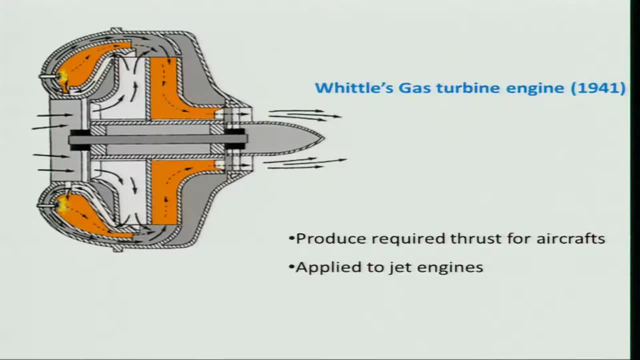 to be known as a co inventor of the gas turbine engine, which was due. but he was not given because they lost the war And of course at the parallelly to, for winning the war. before that there was a first world war. during the second world war the British were trying hard. 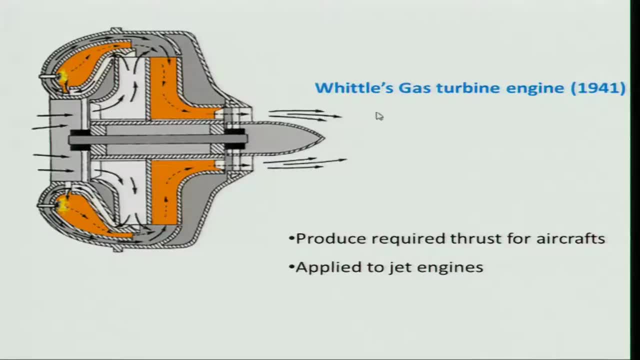 to have a engine and the Sir Whittle developed a engine which I have shown here. In this engine, if you look at, this is your, what you call the third engine. This is centrifugal compressor and this goes into a combustion chamber which I have shown. 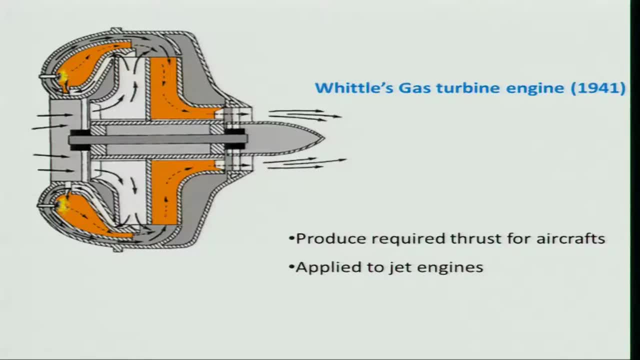 this is known as a reverse combustion chamber, a reverse combustor, And which was quite compact in that. and then it will be expanded in a turbine, which is a radial turbine or centrifugal turbine. of course the nozzle, it will be expanded and you will get the thrust. So, if you look, 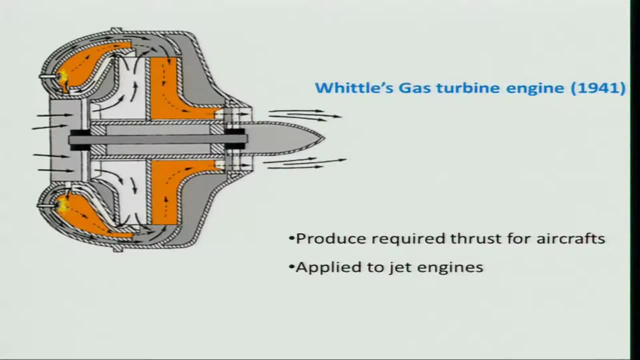 at this. reverse combustor is coming up well Again after lull, and, however, lot of work has to be done on that to have a compact micro combustors, which I would not be discussing about it. However, if some of you are interested, you can look at it. So this is the development of the gas turbine engine, what we could see. 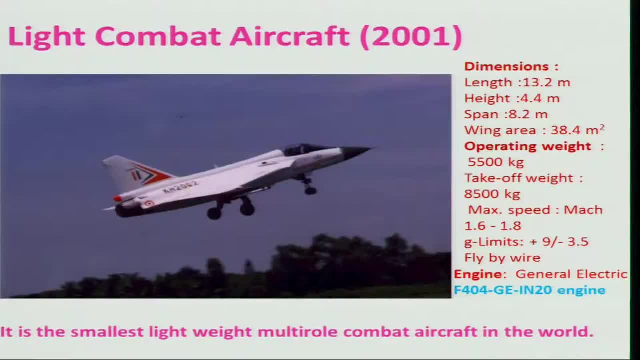 and of course in India we are having a ambitious program of this aircraft engines and also the space craft engine And we could manage to develop a light combat aircraft in two thousand and one and which is basically smallest light weight multi rule combat aircraft in the world whose dimensions 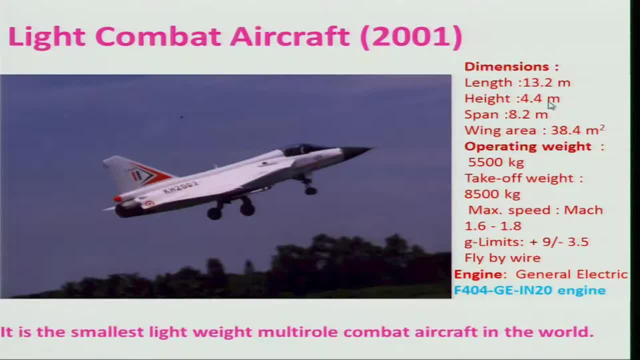 are given and the length is 13. 2 meter, height is 4. 4 and span, of course, the 8. 2 meter. So if you look at, it can cover a MAC number: 1. 6 to 1. 8. it is a technology fly by via. 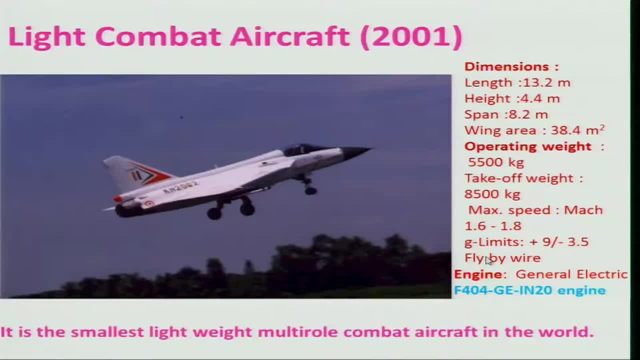 which can cover a m. a can fly various shapes And then they are. Carney cannot produce like 11 am haunting muscle frame at hundreds of miles per hour And you can understand, can, where. and of course the gravity limit is 9 plus 9 g to minus 3.5 g. and keep in mind 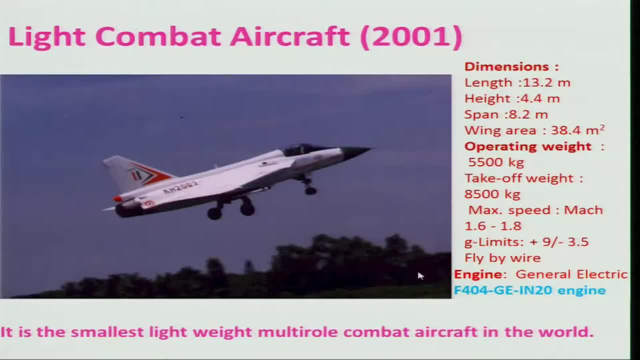 that we are yet to get a engine of our own and this light combat aircraft being propelled or being powered by the general electric F 404 and G E I N 20 engines, And you must be aware that we are having a research establishment known as gas turbine. 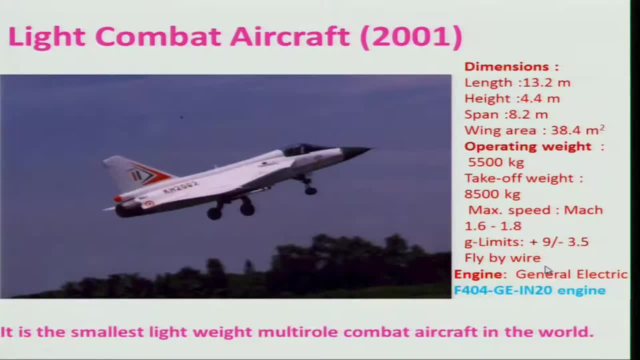 research establishment G T R E, which is instrumental in developing a engine. Unfortunately, we are not very successful, in spite of lot of money being spent. I wish some of you will contribute for the development and it is a important to have such kind of engine not. 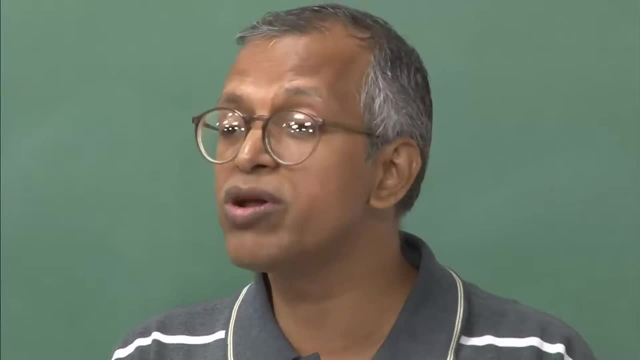 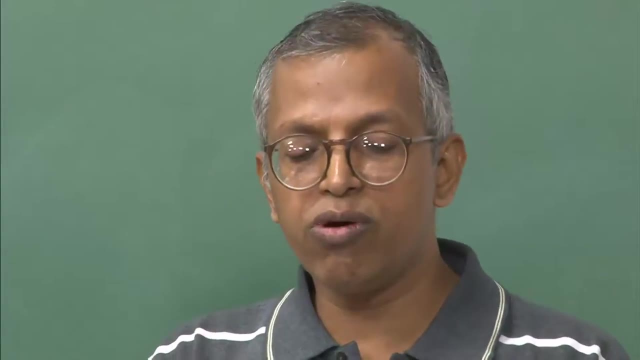 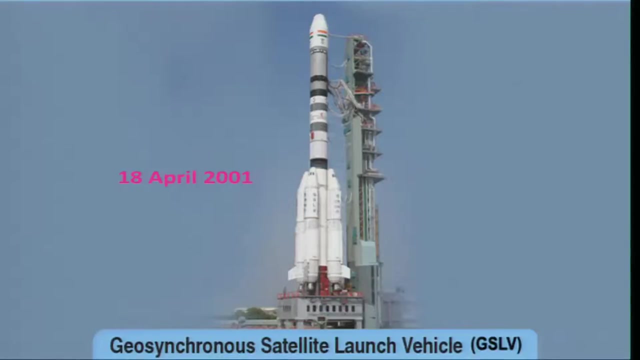 only for having a combat aircraft or, but it is also required for civilian aircrafts and other applications. So we need to augment our technical know how's and knowledge to develop certain things which will be useful. So, beside this, we are having a plan, what we call ambitious programs of launching vehicles. 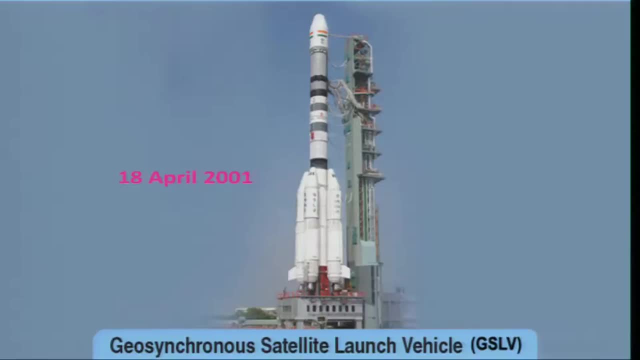 one of them, which I am showing here, is GSLB, which all of you will be aware. this is geosynchronous satellite launch vehicle which was developed in 18 April 2001.. There are several versions which have come up till now, because already 11 years ago it was developed. So this is. 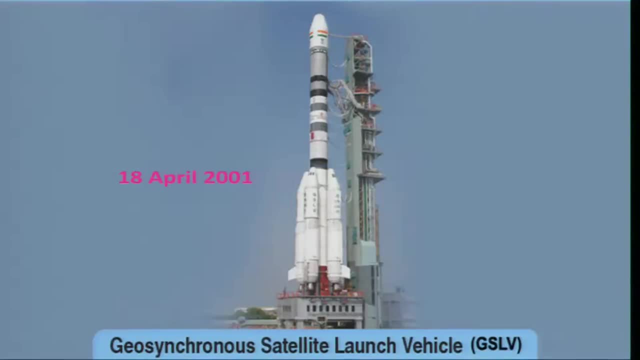 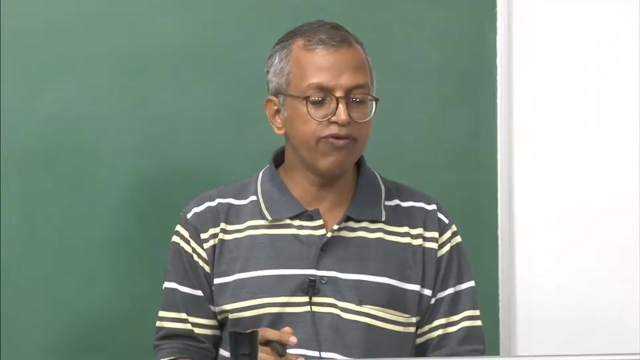 already 11 years or over by this time and which will be, if you look at it, is having a four strap on motors and each is having a booster rocket engines, and there will be first stage and second stage, which will be discussing little later on. but just to give, 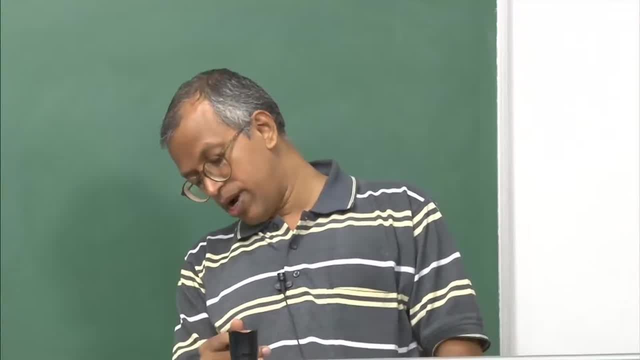 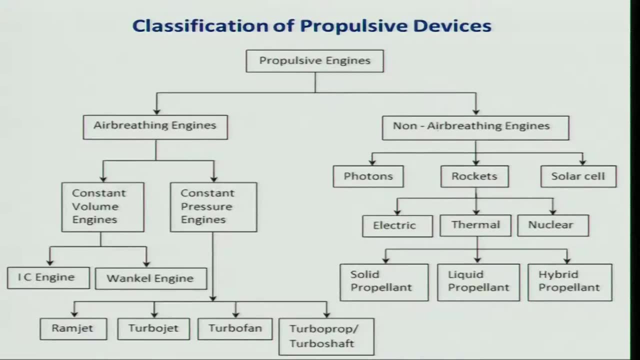 a brief idea. I am just talking about it Now. having come to this brief history of the propulsion, Let us look at how we can classify A propulsive device. as I mention earlier, that propulsive device can be broadly classified into two. one is air breathing engines and other is non air breathing engines. Air breathing- 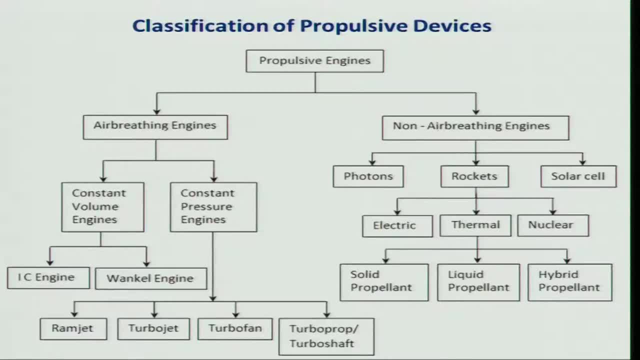 engines means is basically the which will breathe the air. this is the air breathing engine. that means it will be taking air as an oxidizer And you can use as a fuel engine. You can use as a fuel like your piston engine, gas turbine engine and other place, but however, 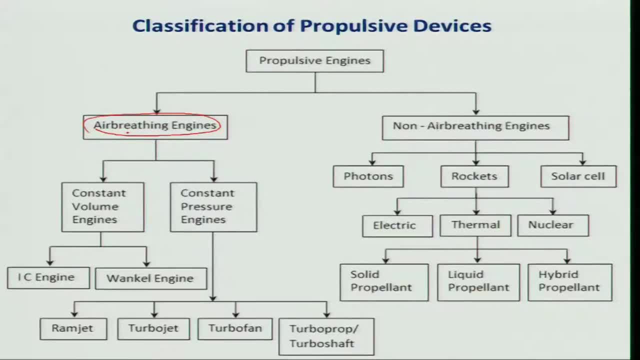 this can be restricted into the what you call in the atmosphere only. but when you want to go beyond atmosphere, naturally you do not get the air, because atmosphere would not be there. and air is not there means oxidizer or oxygen would not be available. So therefore, 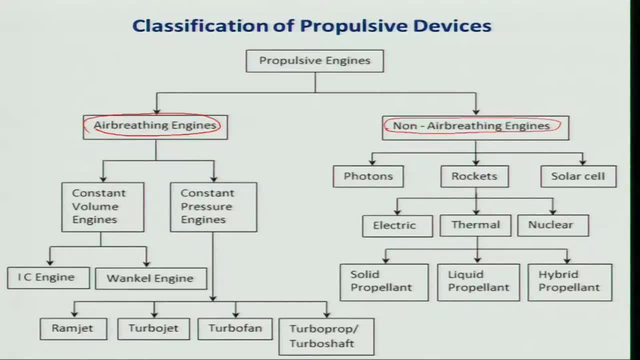 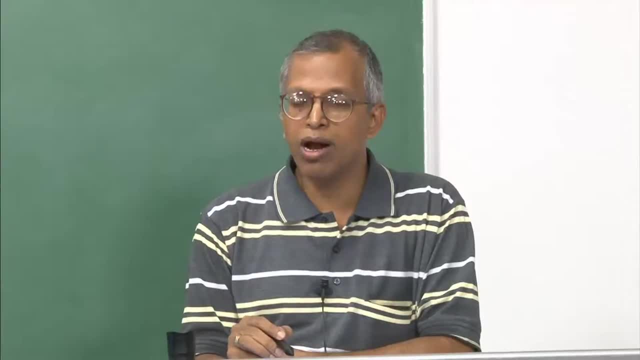 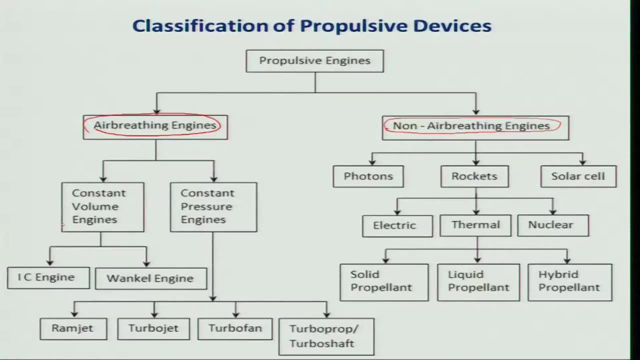 we will have to look at a another class of engine for aerospace application, That is, the non air breathing engines, means it will be carrying not only the fuel but also the oxidizer. So this air breathing engines can be broadly divided into two categories. 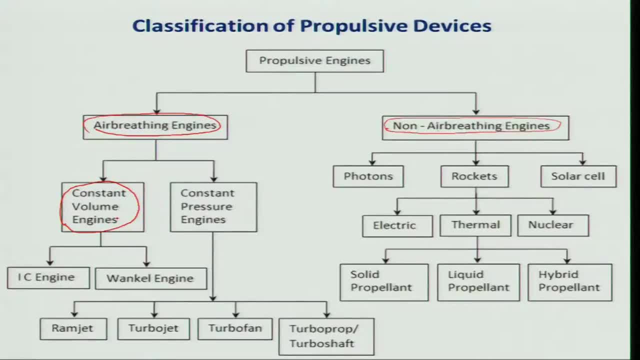 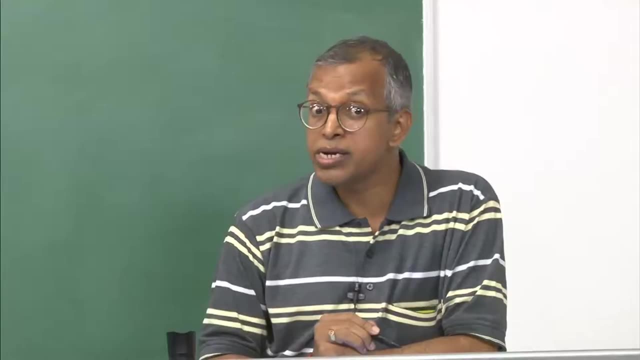 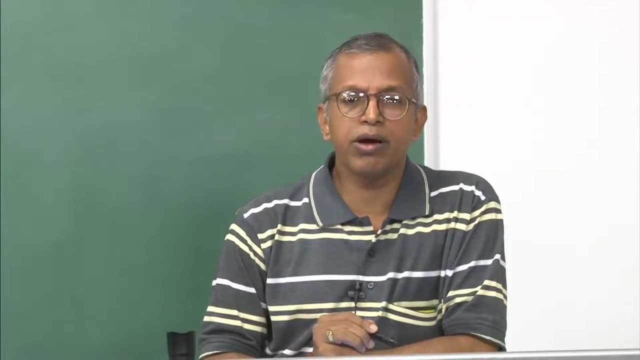 one is your constant volume engines. And what is the example of constant volume engine? like your piston engines? right, it is. it can be spark ignition engine, it can be What we called compression ignition engine or the diesel engine. there are several other varieties, like telling engines, and then your braton engines can be use. br歡 cycle can 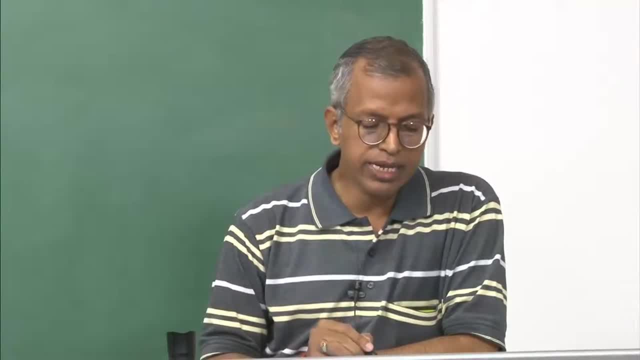 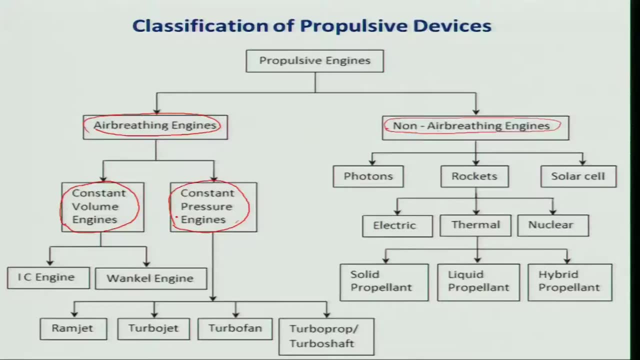 be used in the piston, as is told, But it is not being use. how about? there is another claus of engine which is known as constant pressure engine. what is the meaning of constant pressure engine? during this� kommersiën process, pressure will be remaining constant. 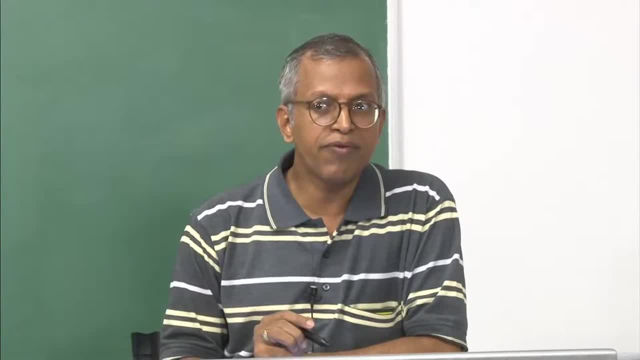 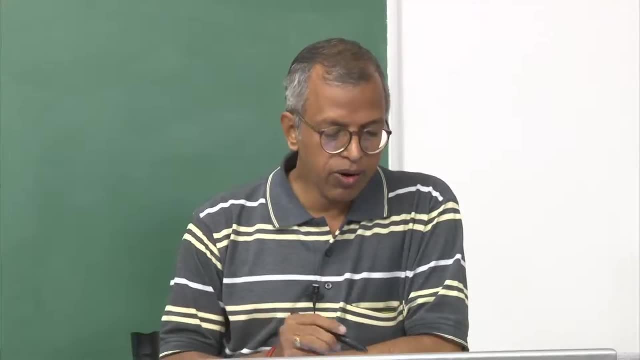 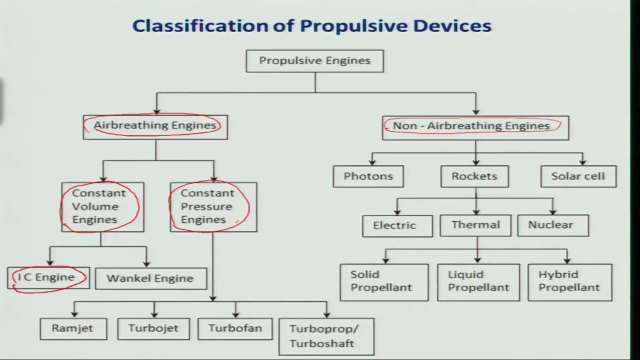 right. How that possible? that possible, that is a matter of you know discussion. we will do that whenever we will get into that. Now let us look at how this constant volume engine can be divided into the I C engine, that is, the internal combustion engine. that is another class of engine which 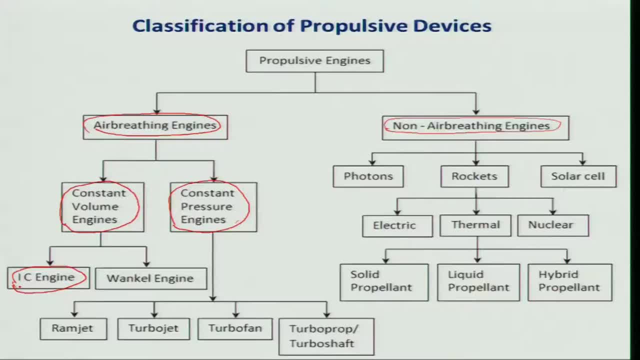 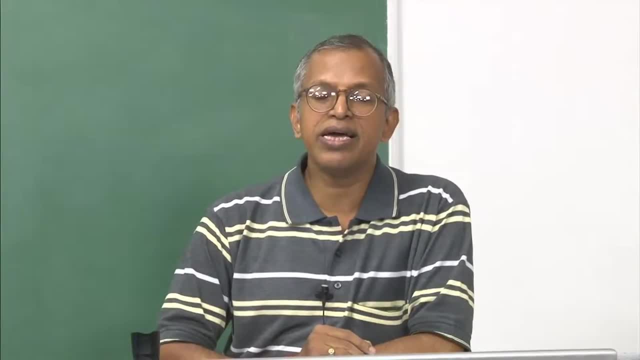 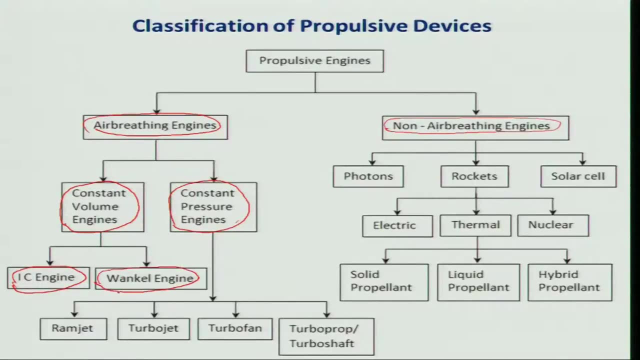 you call it as a external combustion engine. However, for propulsion we do not use it. internal combustion means the combustion will be taking place inside the engine itself. And there is a another very compact engine which I will be discussing little bit is known as Wankel. 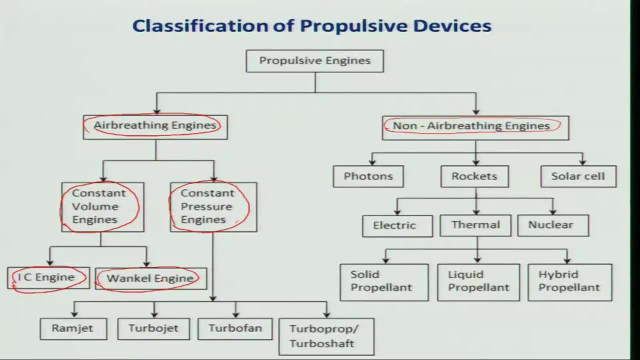 engine which is not being used very much. However, it has a potential to be used for several aerospace applications, particularly air breathing engine class. Whereas the constant pressure engines is divided into two classes. It is divided into the ramjet engine, which will be discussing to some extent very briefly. 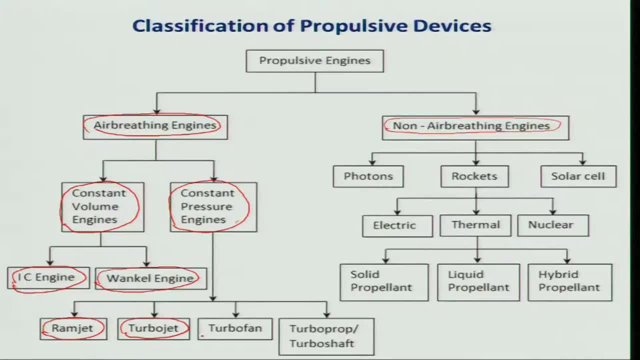 little later on- and turbojet engines, turbofan engines and turboprop and turboshaft engines. So all these things will be discussing as you go along. Let us look at how we can classify this- non air breathing engines- and it is can be divided into three. one is photon engine. 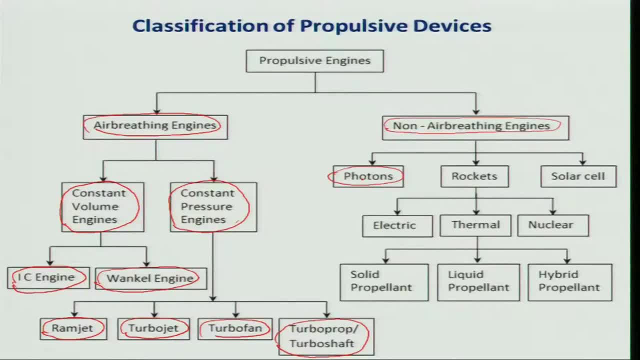 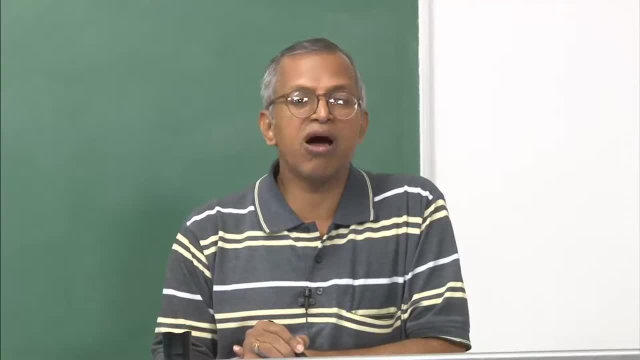 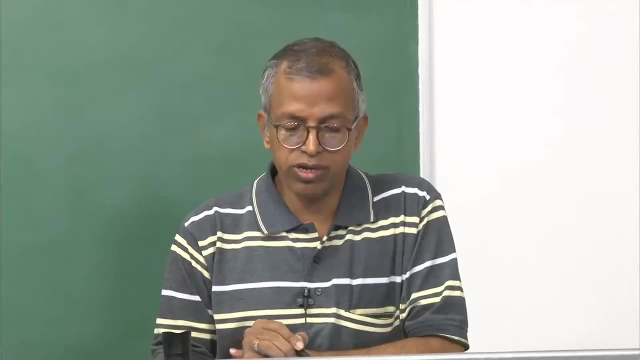 means photons. That means photons, you know light particles and which is basically will be collected in the outer space and can be used, but this is not in a very what you call developed stage. rather I would say that it is very in fancy stage. And there is a solar cell which is similar to that of photons. but however it will be. 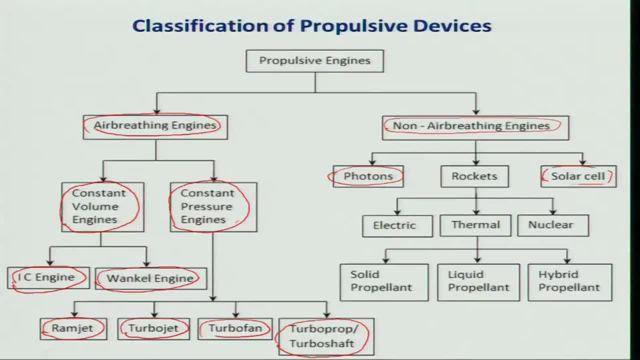 having a panel which will be collecting the photon from the sun and then converting into the various forms of energy, whether it is a what you call solar cell or it can be any other thermal kind of things. What we will be interested in basically the rockets engines, and these rocket engines will be divided again into electrical and thermal. 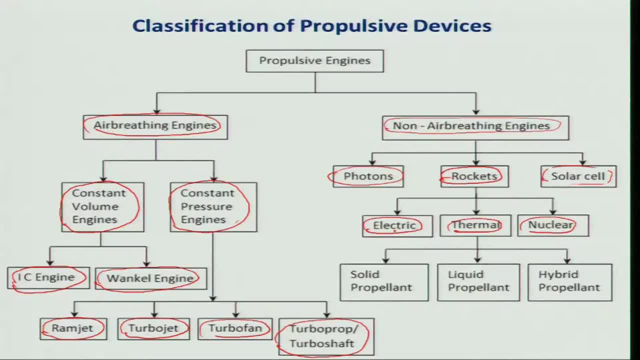 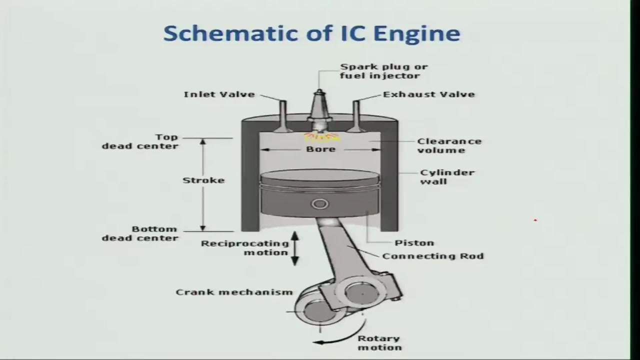 and nuclear. That means electrical energy will be used in the electrical rocket engines, which I will not be discussing. So in the combustion there will be ignition with the help of spark plug and then the combustion will be taking place, which will be pushing the piston, and thus the power will be generated. 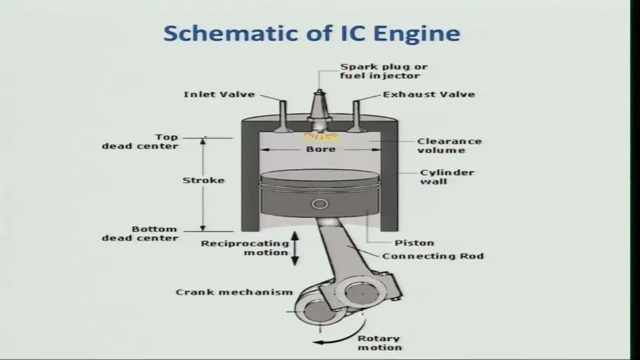 and that is known as power stroke, during which the piston will move from top to the bottom dead center. And then, when the piston will move from the bottom dead center to the top dead center, the combustible, or the, what you call the exhaust gases, will be going to the 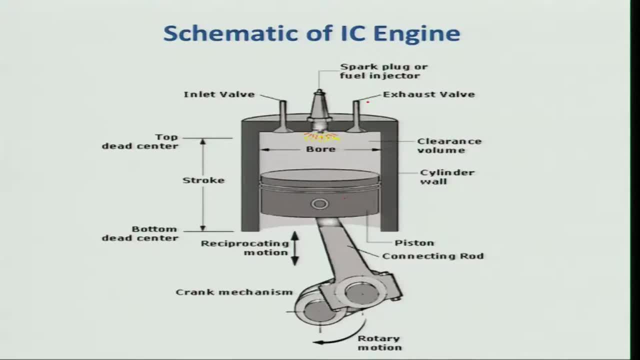 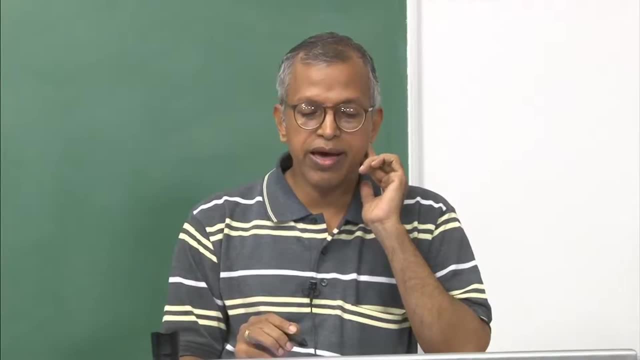 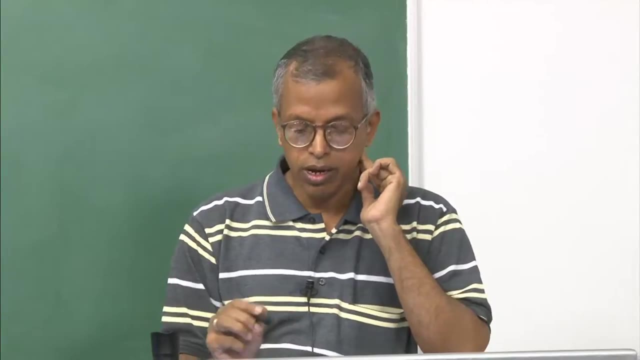 piston going out through this valve and that completes the cycle. Of course, this is known as the four stroke engines, but however there is a two stroke engines which is being coming up again. it can be utilized in future And unfortunately I would not be covering in this. 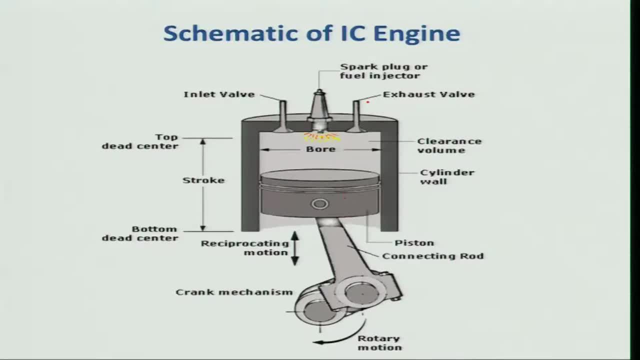 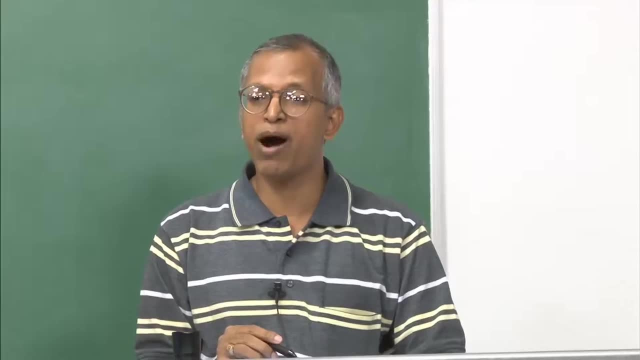 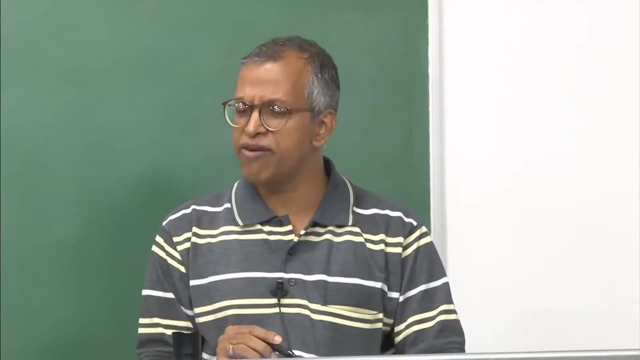 course, the piston engines as such, although a large number of aircraft, even today, if you look at the number wise- Are being powered by the piston engine, and in our flight lab we are having seven aircrafts which are being propelled by the piston engine. Therefore, I would ask you people to look 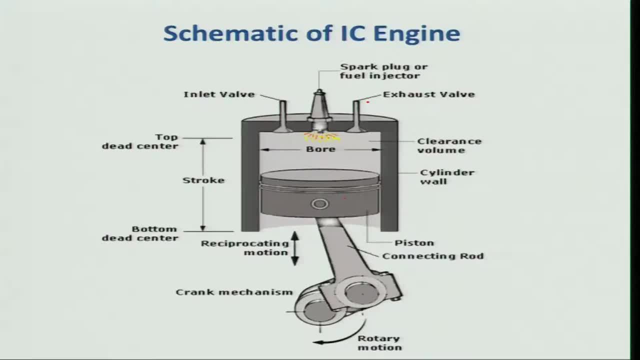 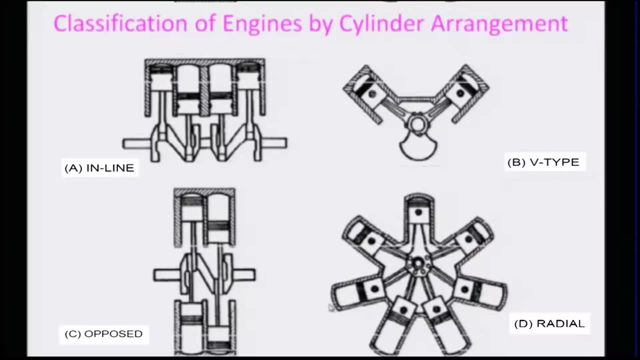 at it and learn yourself, and may be some of you can write a term paper on piston aero piston engines, which is different than the automobile Based on the cylinder and piston arrangement. we can classify the engines into what we call the four, but of course you can have more, but here I have shown the four type. one is: 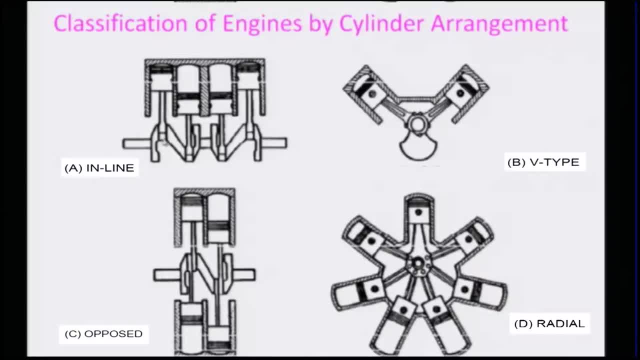 in line engine, if you can look at, there are several piston cylinders are connected to a same crank shaft but with different phases, phase angles, such that it can move tandemly or move in a continuous manner without much fluctuation in the power level on the load. 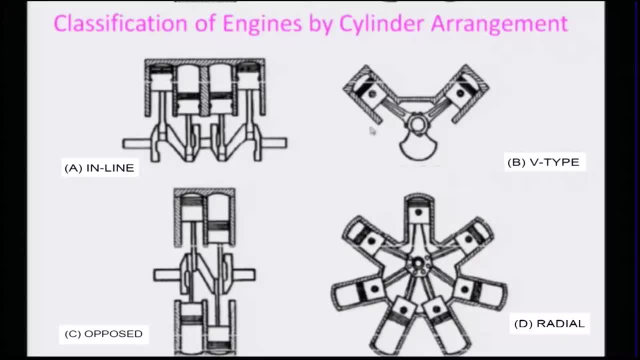 on the crank shaft, And the another kind is the v type, v type and which is piston and crank shaft being connected through this to the shaft in such a way that it will cancel each other along this what you call horizontal force, So that 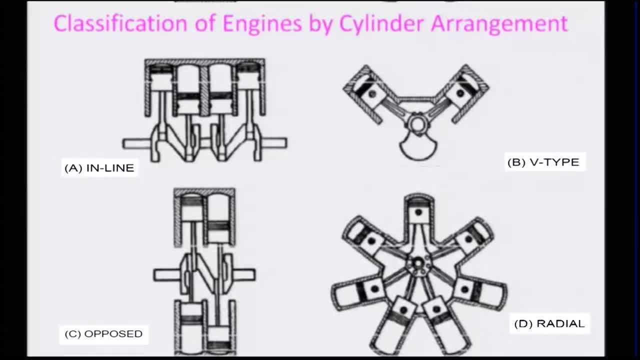 the balance will be better. and there is another oppose piston arrangement, which is shown here, that both the this pistons like are opposing to each other. For example, this is at the top dead center, these are the bottom dead center kind of things, both the vertical it. 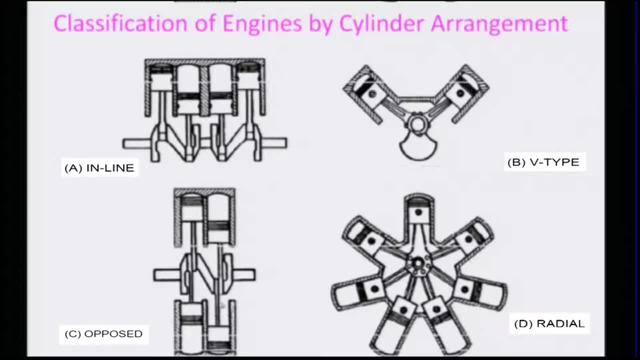 can be what? vertical, and it can also be horizontal. The basic idea is that the shaft should run smoothly and without this thing, but this is not really being very much use in air kept engine. however, in line and v types are being used And so also the radial. in the radial, the piston and cylinder are being arrange along the radius. 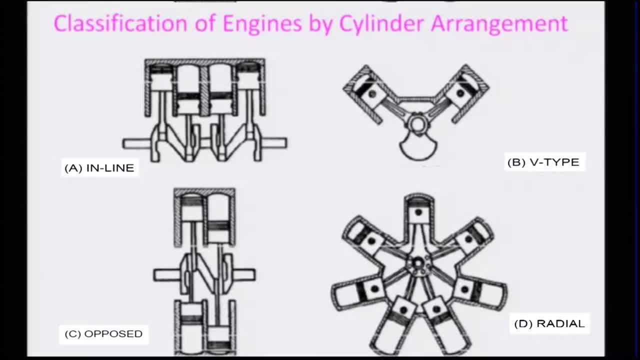 such that The it will be, the power will be transferred to the shaft in a very smooth manner without much fluctuation on the load and other things. So we will be discussing a little more in the next slide, that is in in line and radial, which are being used very much for the aircraft. 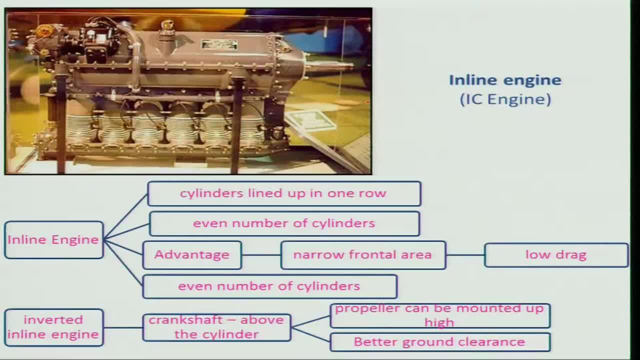 engines. So under this category I will show you two engines. one is in line engine, as I told that, it is being used by the ride brothers and which is having a cylinder. These are the cylinders which is lined up in one row and, if you look at generally, piston on the 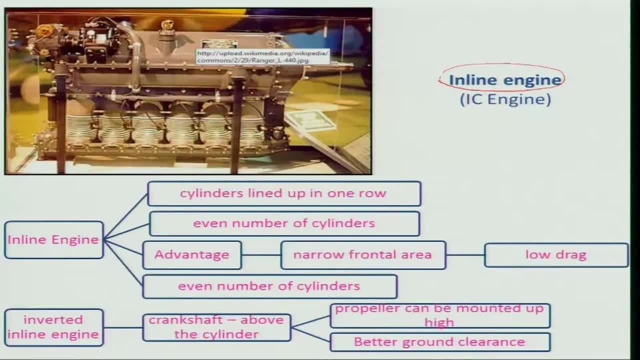 top, but here, in this case, pistons are in the bottom and this is the crank shaft, which is having a shaft, which is shown here and to which the propeller will be mounted. and this is being done because of propeller can be mounted easily and better ground clearance. 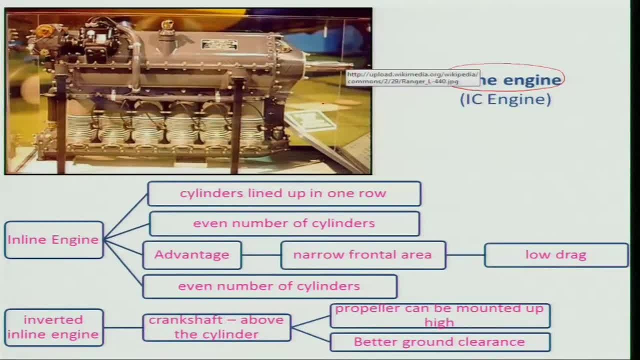 you can have. size is higher, So you can test it well and put it. So, therefore, this kind of engine which is being used and it is having a narrow frontal area and lower drag, can be. therefore it is being used in the engines And of course there are several V engines, which is together. 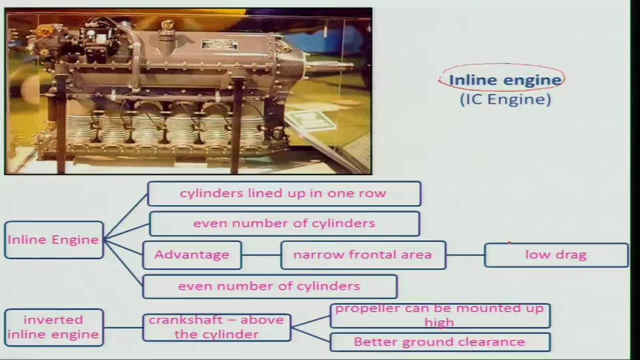 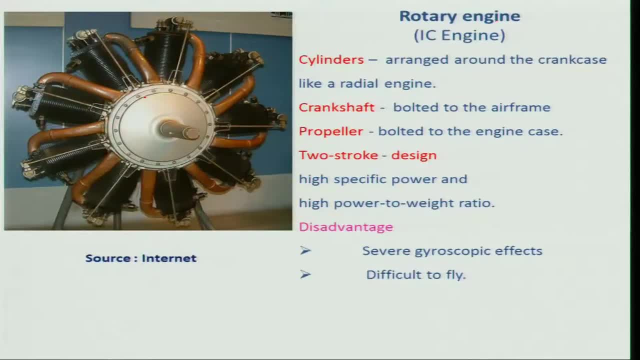 being used, and there is another engine which you can see in our flight lab which is being kept as a model. I guess it is a rotary engine. That means the cylinder. these are the cylinders which are being mounted along with the thing and, as a result, it will be well balanced right. 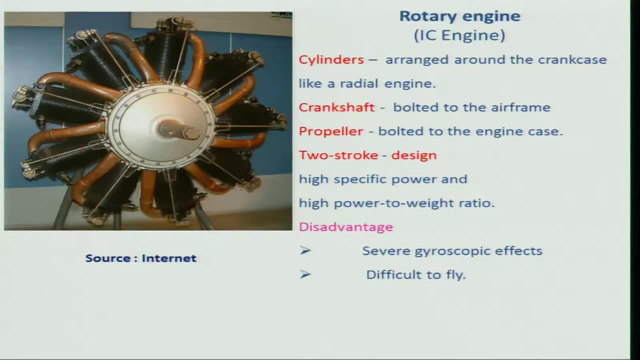 The balancing is a big problem in the iso engine, you might be aware. those people who have studied the mechanical engineering will be knowing that. So it is a cylinder arrange around the crankcase like a radial engine and it is a bolted. the propeller is bolted. 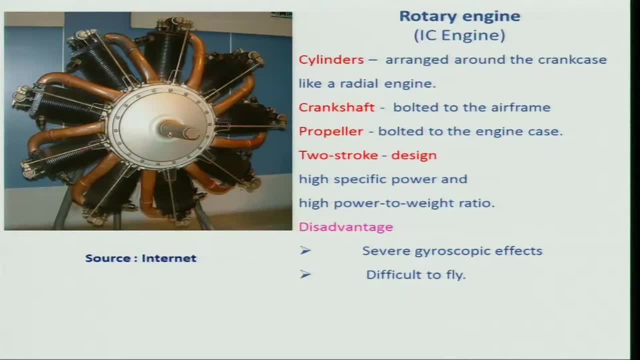 to the engine. So this is the place where it will be bolted and it is a generally a two stroke design. as I told, that engine can be four stroke and two stroke. it is having a higher specific power and high power to weight ratio. Of course, there are several disadvantages that severe. 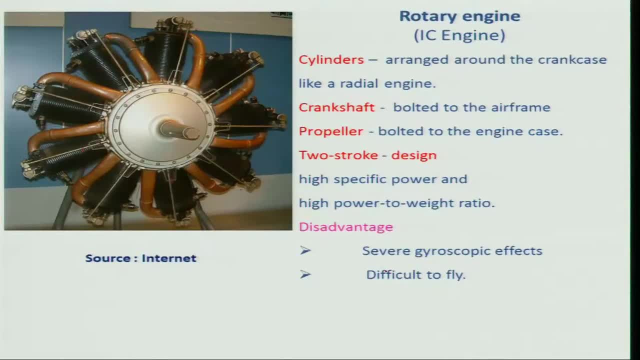 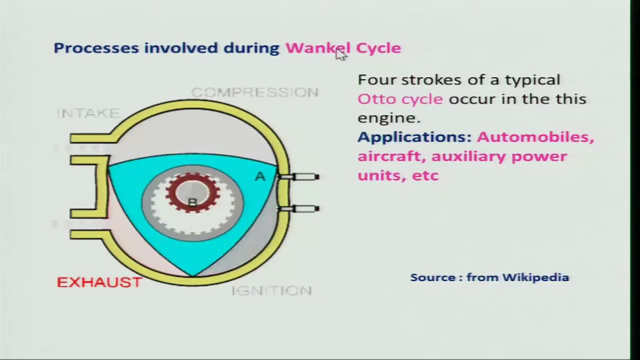 gyroscopic effect and difficult to fly because it is little bit heavy in nature. So it is not being used now a days. however, it was being used earlier days. Now I will be discussing about Wankel engine. I am very much fascinated by this engine because 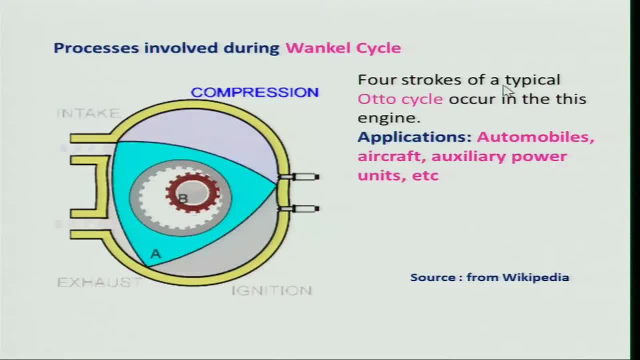 it is quite compact. It works on a basically four stroke of a typical auto cycle. in this engine you can look at this animation that air is coming over this known as air intake. it will be compressed and then, once it compressed, then the ignition, the combustion, take place. 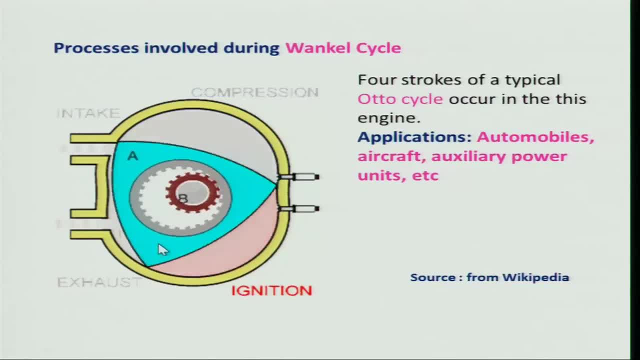 over here, Then it will be expanded, it will be going to the exhaust. So this is a quite compact engine and, of course, lot of people, lot of research groups across the globe are working and in India, NAL, that is, national aeronautical laboratory, is working on this engine for a quite some time and I 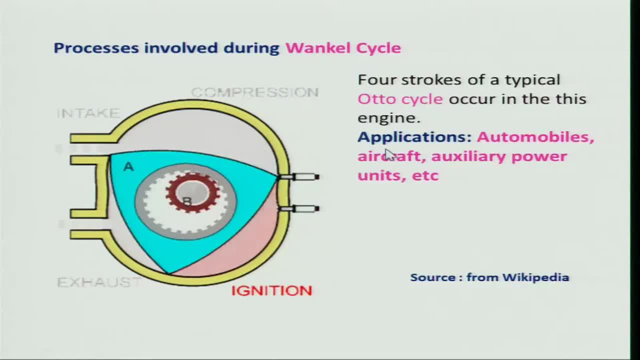 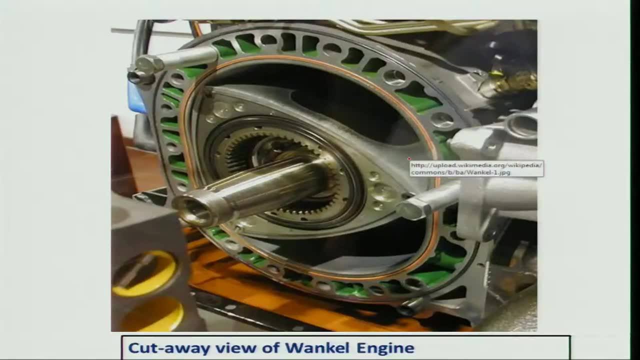 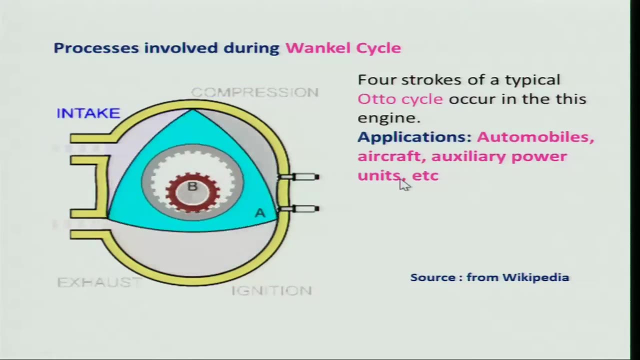 was told it is in operational mode at this moment. This Wankel engine can be used not only for the aircraft, but also for the what you call the automobile and auxiliary power units and other things. So I will just show you a cut away view of 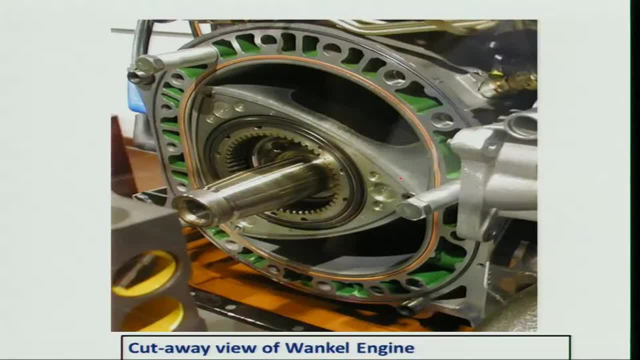 the Wankel engine. it looks to be quite simple as compared to that, but it is a quite compact as a at the same time. And if you look at these epileptic gears and this is the chamber where The combustion, and then you know air will be coming inside and then it will be reacted. 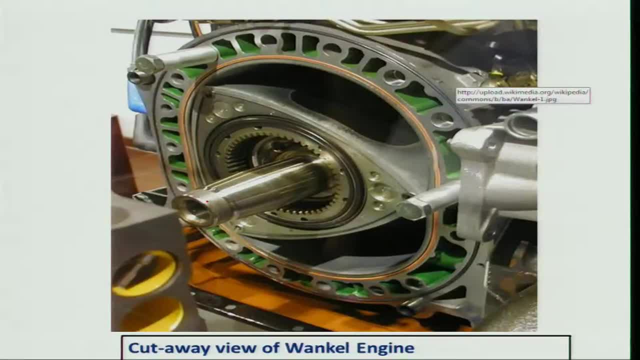 somewhere here igniters and it will be going out. So this engines is a quite promising one according to me, but unfortunately it has not been used in real situation. I hope and wish that it will be worked. may be some of you will be looking at it if you are having 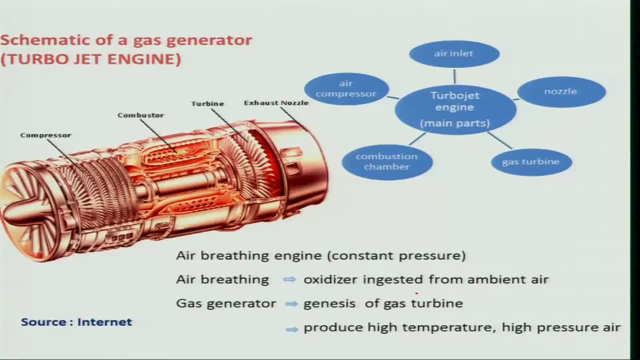 interest in engine like this. So let us look at a A gas turbine engine. that basically it is a gas generator, which I have shown here. This having a compression is having a combustion chamber and this is having a turbine, and this constitute the gas generators. And whenever the gas generator is connected with a nozzle, 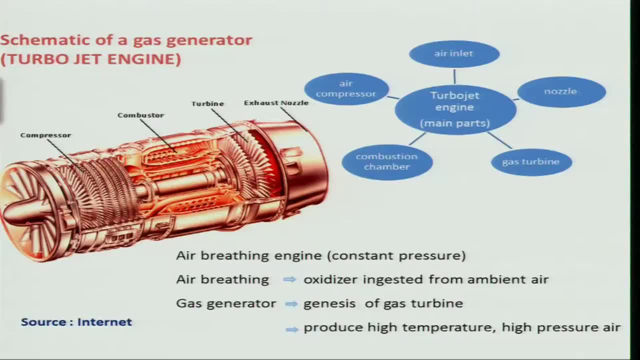 and an air intake which is not shown in this figure is considered as an aero gas turbine engine or turbo jet engine. right So, as I told you, this is a air breathing engine and the combustion takes place in this place, which is at a constant pressure, right that? 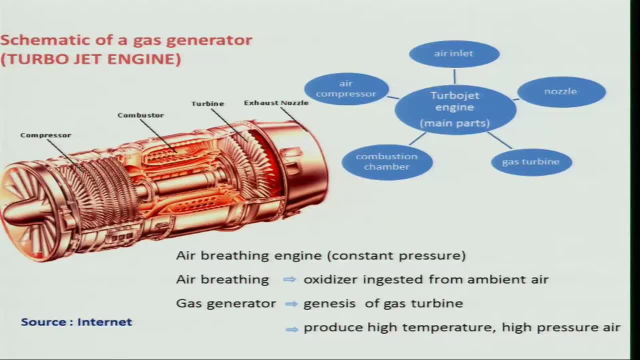 is why it is known as constant pressure engine. And, as I told you, what will be happening here? when air will enter into the air intake? there will be increase in pressure because the kinetic energy is converted into pressure energy, and then You further compress in the compressor and there is a combustion chamber where the heat 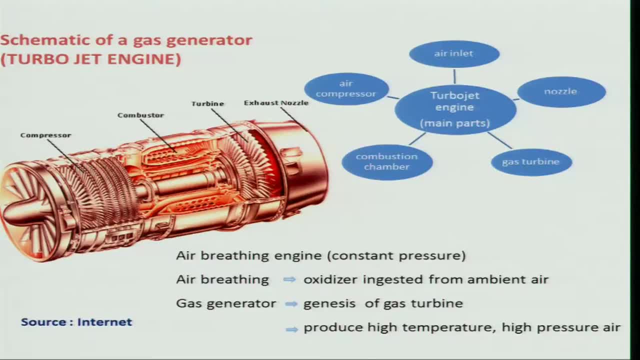 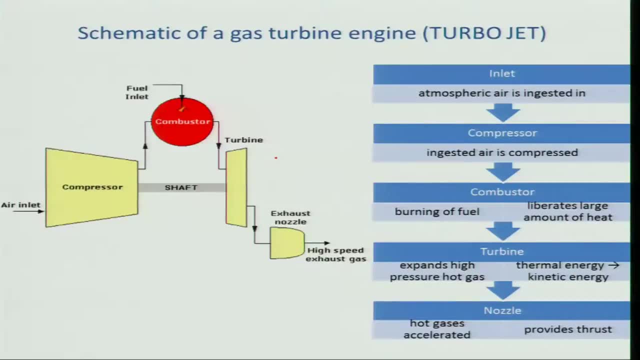 being added and the. it will be expanded in a turbine and it is expanded further in the nozzle to produce the thrust. So if you look at, I have shown the schematic diagram here. there I have showed you a cross sectional view, which is air will be entering into compressor. 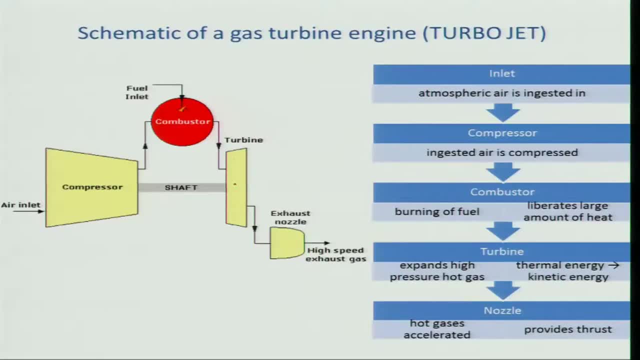 and this is the combustion chamber And the turbine. keep in mind that turbine will be producing power, which is just mean to run the compressor. it would not be giving you any thrust And of course the thrust will be obtained by the, by expanding the gas in. 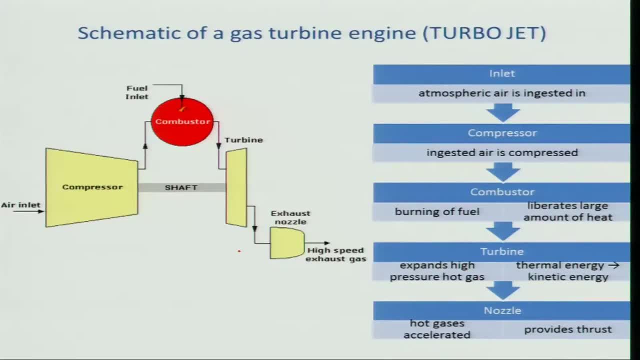 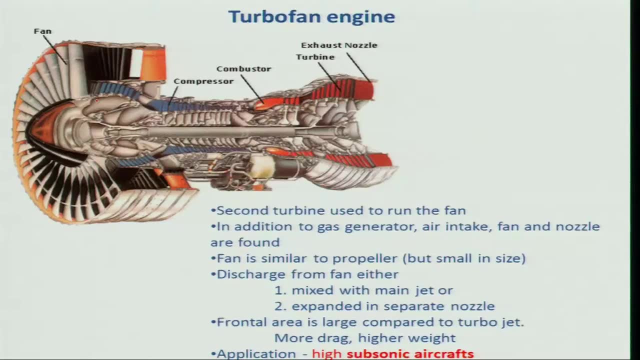 the exhaust nozzle. So that is a basically what you call the turbo jet engine, and there is a another class of engine which we will be discussing. but let us look at a cross sectional view which is similar to that of the turbo jet engine. 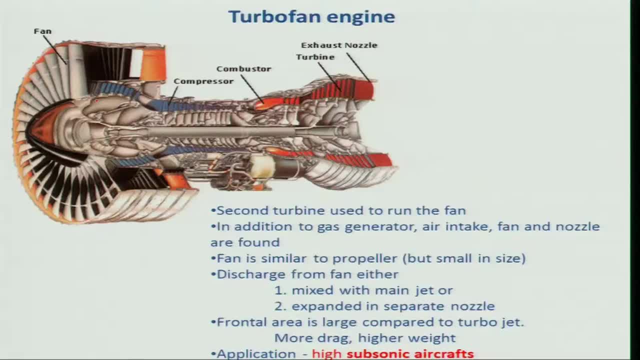 The turbo jet engine. however, it is having little difference. that is, apart from the core engine or the gas generator. it is having a big fan and also a nozzle, And this we can also nozzle when it is expanded. the gas going through the fan it can produce also some thrust. 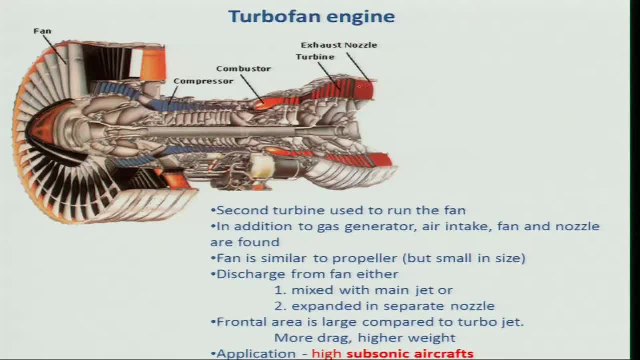 And beside this there is a nozzle, exhaust nozzle, in the core engine which will be producing the thrust. So total thrust by the engine can be obtained by both the fan nozzle and the exhaust nozzle, and there might be a situation where both the fan stream and the core stream mixed together, Then can be expanding. there is a various varieties. 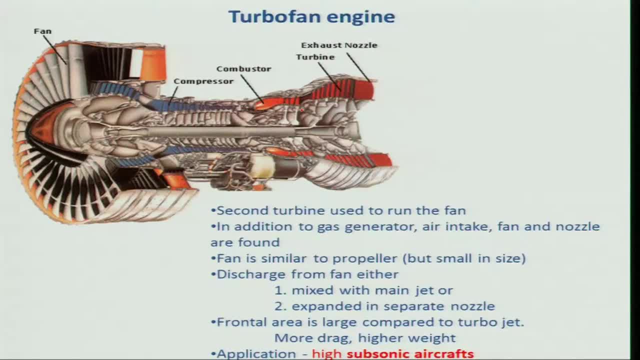 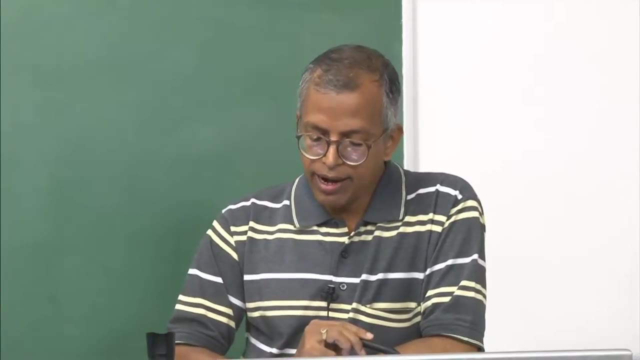 of these turbo fan engines is there and keep in mind that it is being use very much for high subsonic dir website to turbo jet engine. However, it gives a lot of drag as well as compared to the turbo jet engine engines. So what are the advantages and the what you call disadvantages we will be discussing? 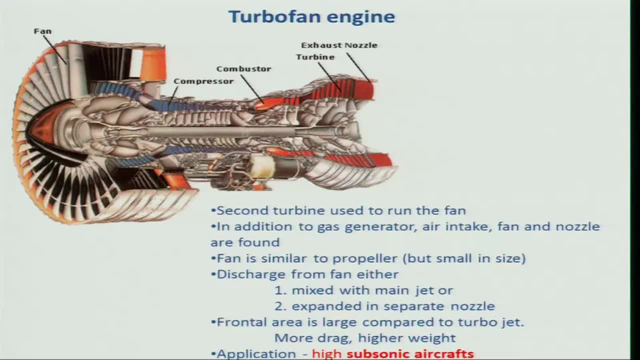 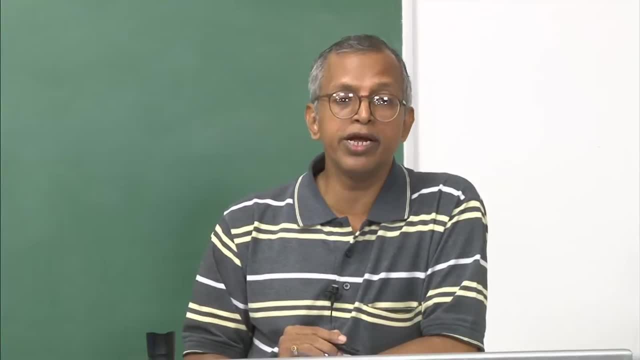 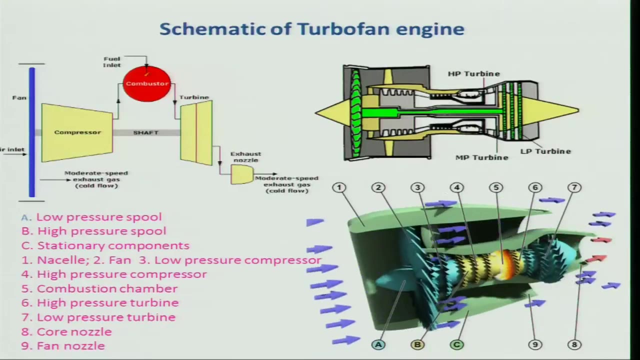 little later, but keep in mind that it is a heavier than the turbojet engine. it is having more drag. However, it is being used in the your passenger aircraft or the civilian aircraft like Boeing kind of class. So let us look at now a schematic I have just shown you and 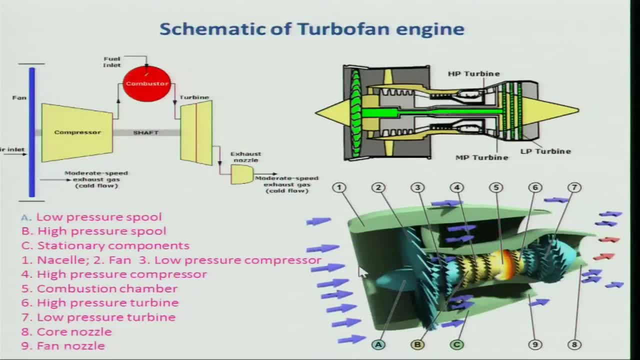 I have already discussed about this thing. you just look at animation. what really happens In this case? it is having a two spool engines. what is the meaning of this two spool engine? one is low pressure spool. that means that is a shaft, which is will be the low pressure. 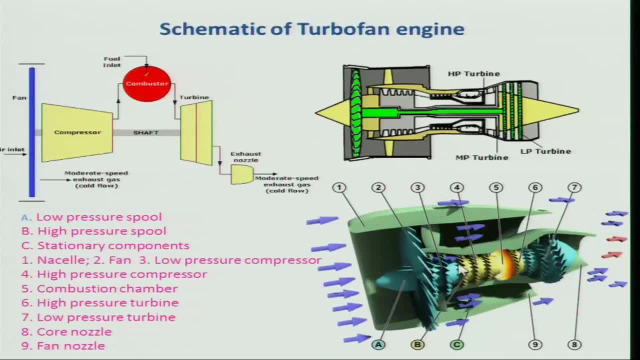 like low pressure turbine, which will be here, you know, will be connected to the your fan, and where the high pressure turbine, which will be somewhere located here, will be connect to the compressor. And then this is having a two concentric shaft which will be rotating. that means two. 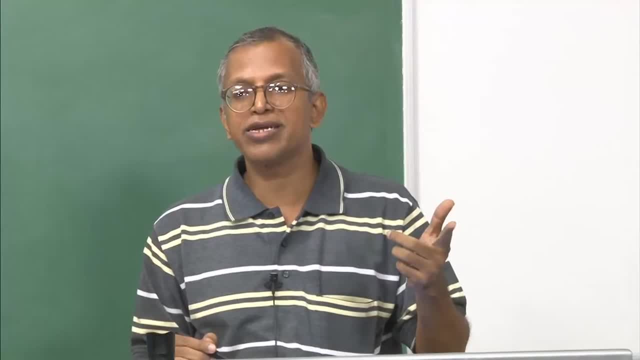 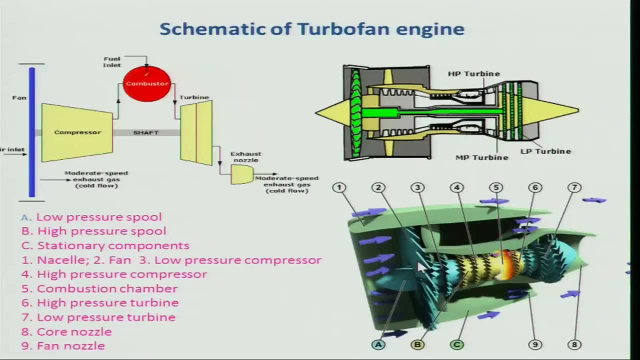 r p m are being used, unlike in a turbojet engine, where the r p m will be one or the shaft will be one, because of fact that the blade- what you call the fan- will be rotating at a lower speed. that is the important. So, beside this, of course, this is the two separate. 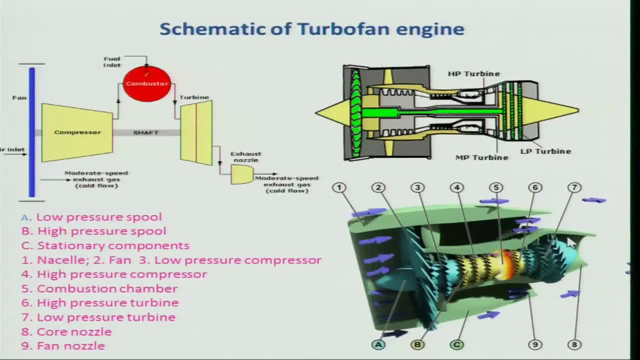 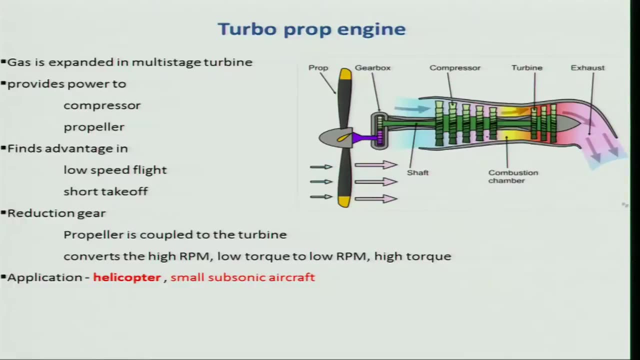 nozzle which I have shown here. one is core nozzle, other is fan nozzle. So now we will look at the turbo- what you call shaft engines, and turbo shaft engine. if you look at it, is having the similar what you call core engines, except that it is connected. 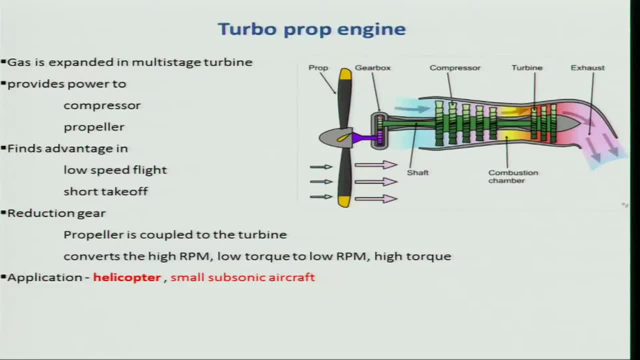 to a propeller through a gear box And this gear box is quite heavy as compared to the you know, like your Engine components. because why it will be heavy. if you look at your ice engine or automobile engines, you do not have a very heavy gear box. why this aircraft engine will be have. 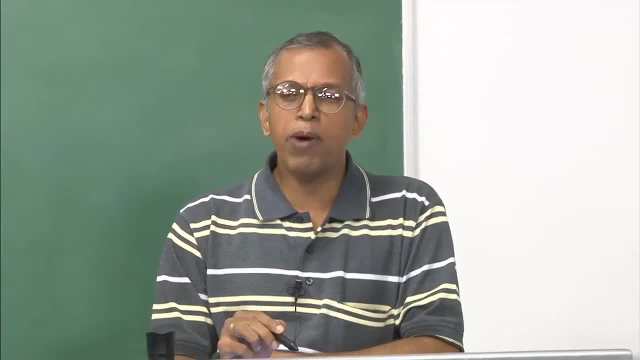 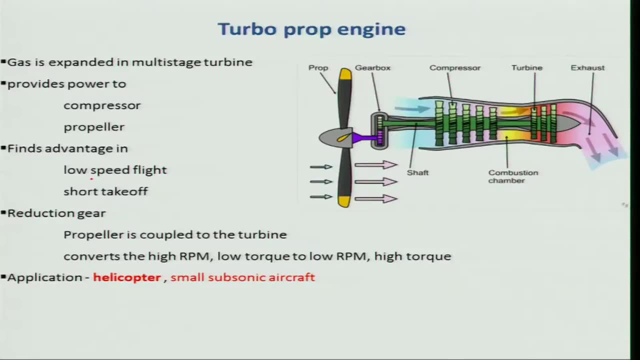 r p m not only has to be reduced, but also the power level will be much higher. So but however, this kind of engines which use find application, low speed flights and shorter take off and also what you call like vertical take off, Vertical take off, kind of things it can do, and it is used in helicopters and small subsonic. 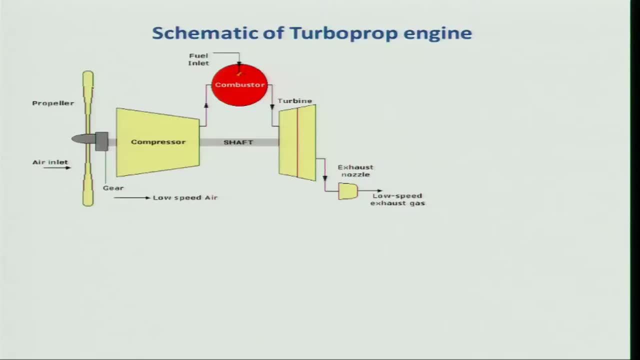 aircraft engines and the schematic I have shown here. it is having a propeller, is having a gear box, compressor and combustion chamber. it is having a turbine, which will be one will be like high pressure will be connected to the compressor, where the low pressure will be connected to the propeller through the gear box. And of course you may get sometimes 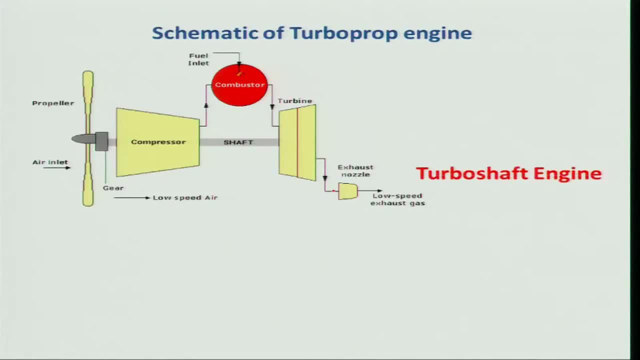 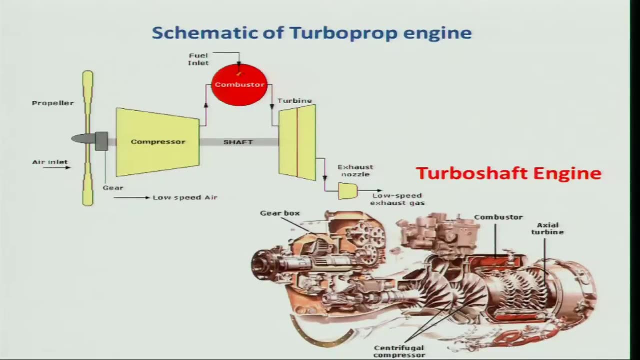 the Thrust through the nozzle, but there is a turbo shaft engine which will be, you know, only whenever you know power will be available in the turbo shaft and no thrust being obtained in the exhaust nozzle as such, And it is having several application, as I told you particularly. 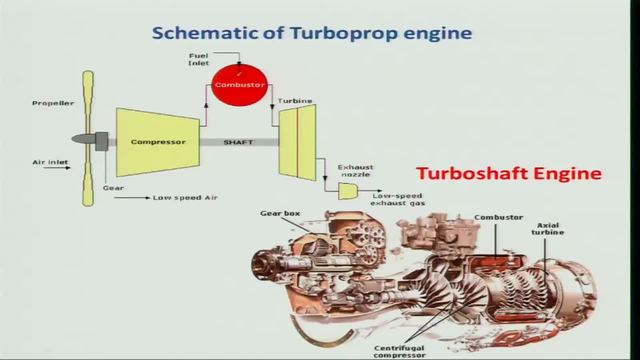 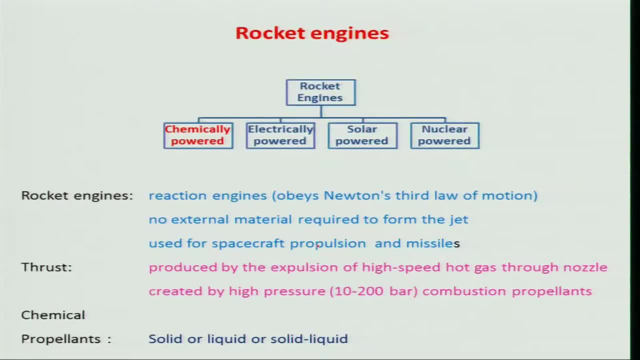 for the vertical take off and short take off and landing. it is being used very much. So let us look at the rocket engines. as I told, that, Rocket engines is basically the reaction engines, which obeys the Newton's third law of motion, and in this case no external material is really required to form the jet. What do 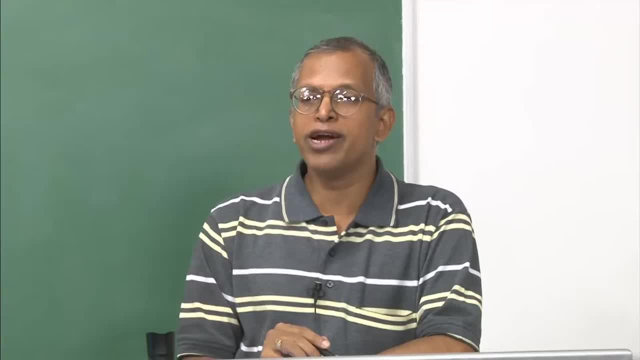 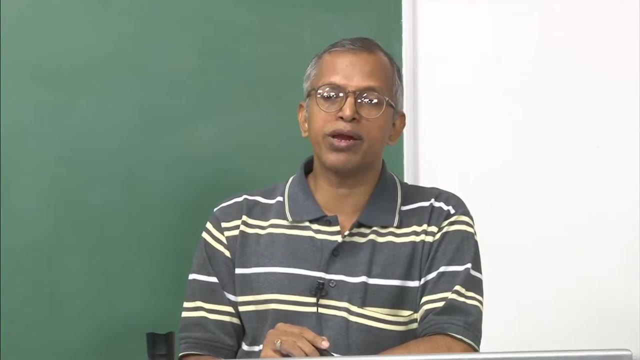 you mean by this external material. basically, you need not to take any air from the atmosphere. you are going beyond the atmosphere. then you need to carry both the fuel and oxidizer such that it will be independent of atmosphere And if you look at the performance of the everything engine will be dependant on the 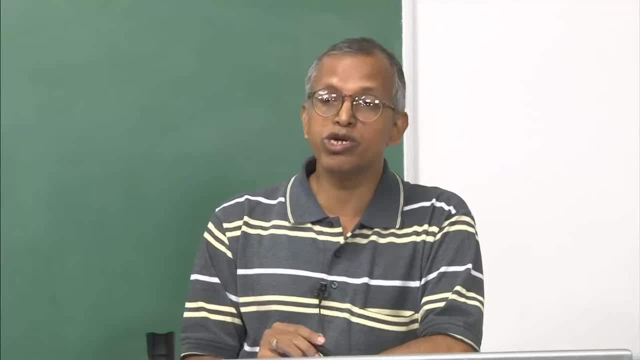 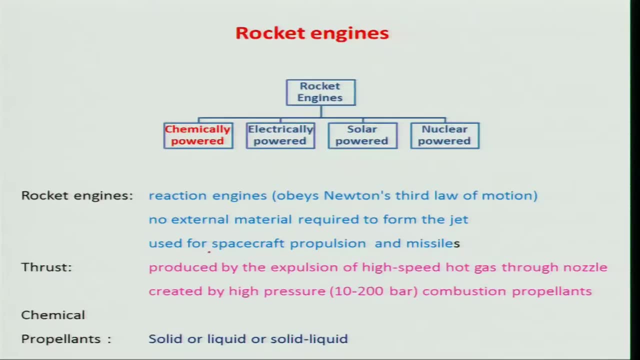 condition and the of the atmosphere through which it will be passing through, whereas it is independent of- And that is the beauty of this- rocket engines, and it is as I mentioned earlier. it is used for space craft propulsion and missiles, and there is a lot of development. however, it 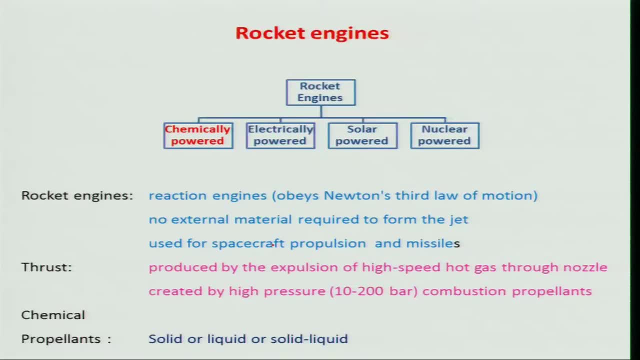 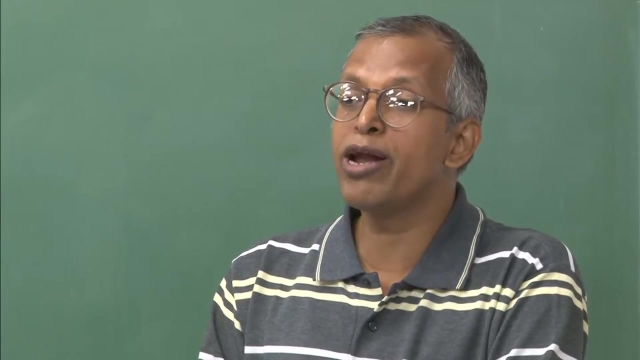 is. but if you look at, we spend A large amount of our budget for the difference in the name of war f, which is a quite a beat, and it is not only in this country but across the globe. we spend lot of money and lot of resources, lot of man powers for winning a war and which is 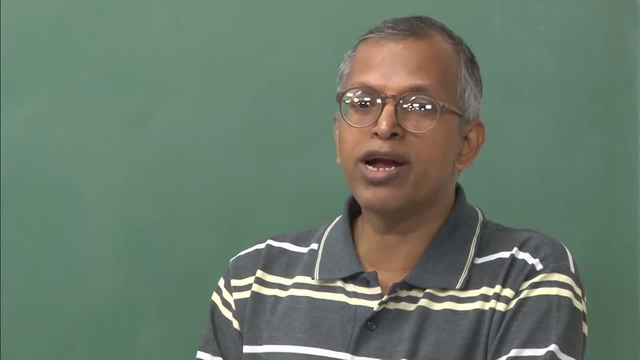 in future. So therefore, it is very important to look at that we should not only be a part of this colossal wastage of resources and see that, how it can be utilized for the elevation of poverty and other things, So that our country 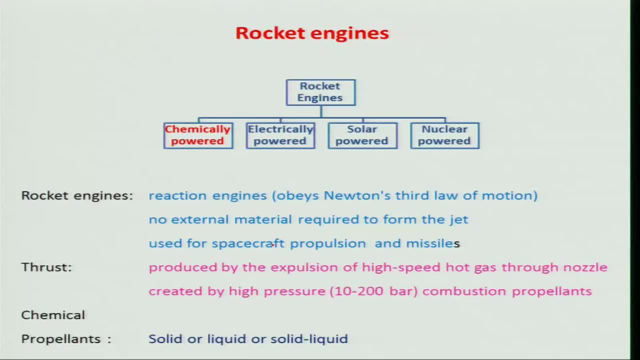 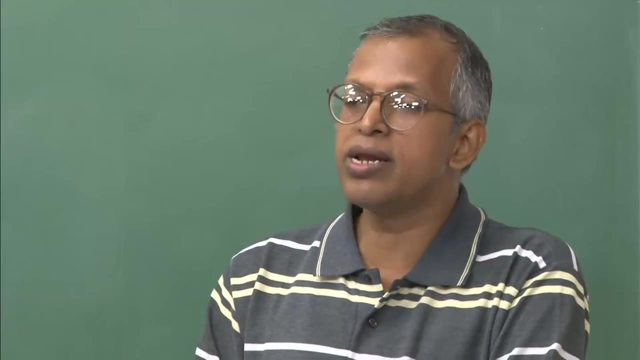 and other places can be leave peacefully. So I must tell you that, although I teach this subject, but however, I feel that it must not be used and abused by this- the war mongering people- to have a war. So, however, there are several civilian application which can be. 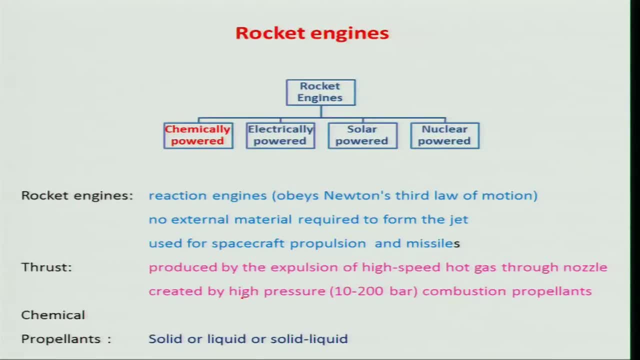 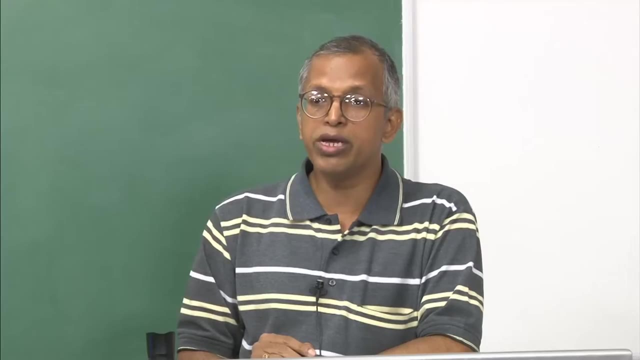 done and which must be done. So use that thing, I must ask, because all of you that, as you people are the next generation or the leaders of this country, technically, man power particularly, and you should see that we should not really look at in a this aspect, rather, use that how we can use for 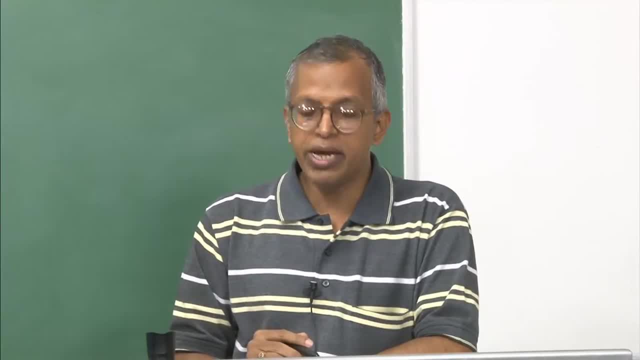 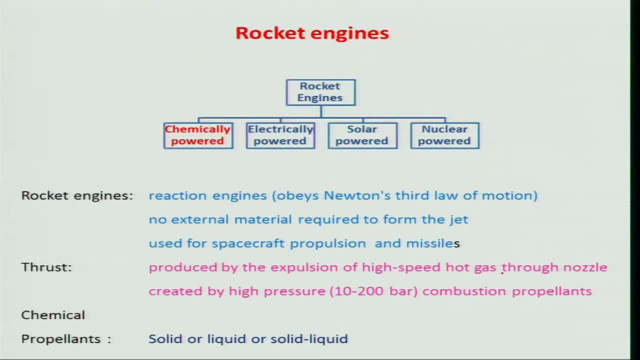 the other, man driven applications, without spoiling the atmosphere. that is very important. So if you look at this, produce the expulsion, high speed hot gas through a nozzle. This is the basic principle Which gives you thrust in case of air breathing engines, particularly class of your turbo jet. 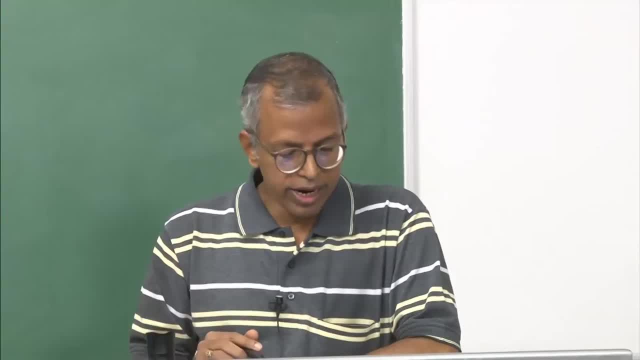 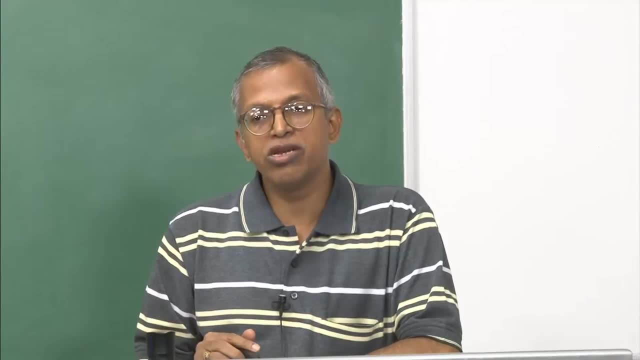 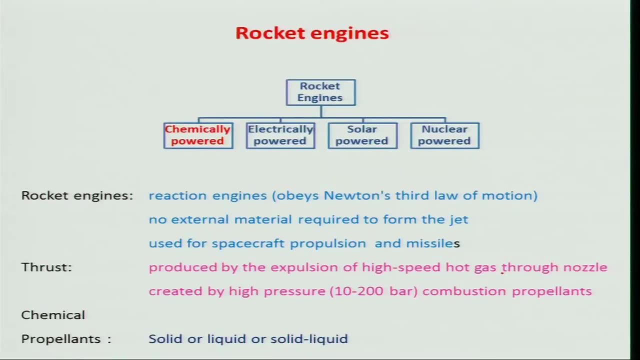 turbo fan and to turbo prop and also the rocket engines, Whereas your IC engine based or the piston engine based is basically through the propeller, And here we use the propellants, which are basically chemicals. and as we are talking about the chemical propellants, 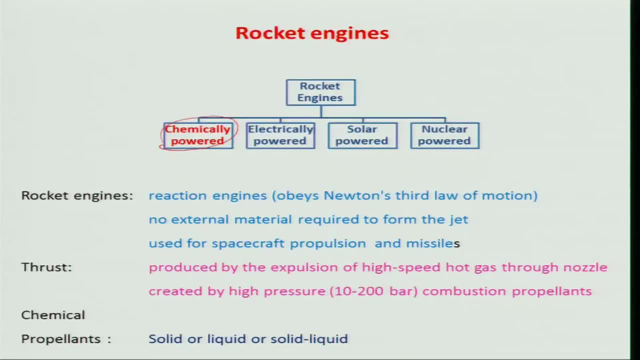 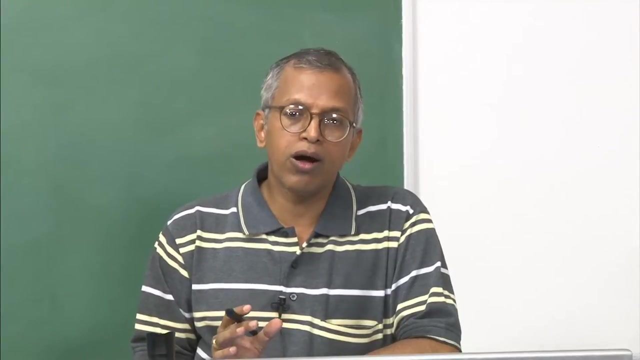 Powered engines and the solid liquid or solid liquid engine, what we call it as a hybrid rocket engines, And we will be discussing little bit about electrical power engines now and solar power engines and nuclear power engines, And I just want to give a bird's eye view of this thing, although this course is focused to on the chemical rocket engines. 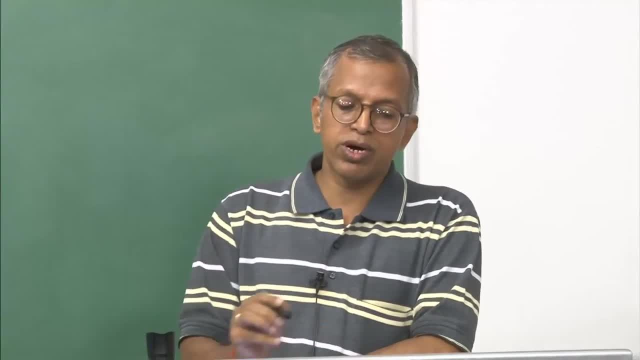 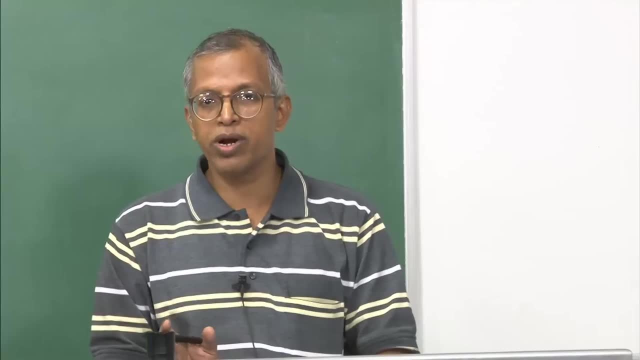 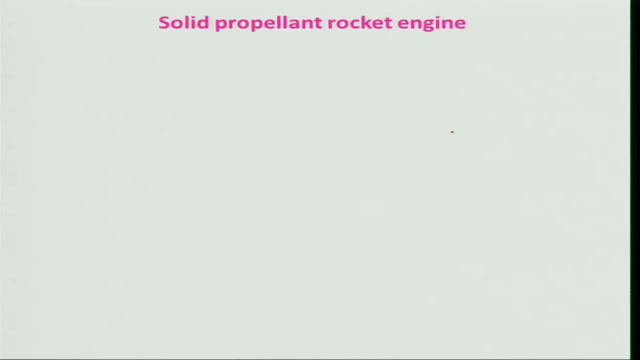 and the gas turbine engines. However, I just want to give a view so that you can get a whole view, but we will be concentrating on the two aspect. one is rocket engine, other is the gas turbine engines And in this course we will be looking at the. whatever the fundamentals are required to delve into the aerospace propulsion. 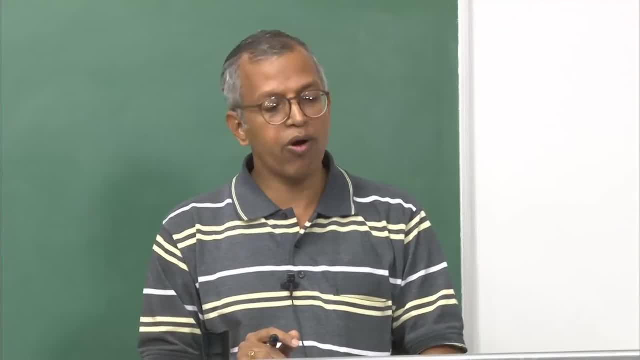 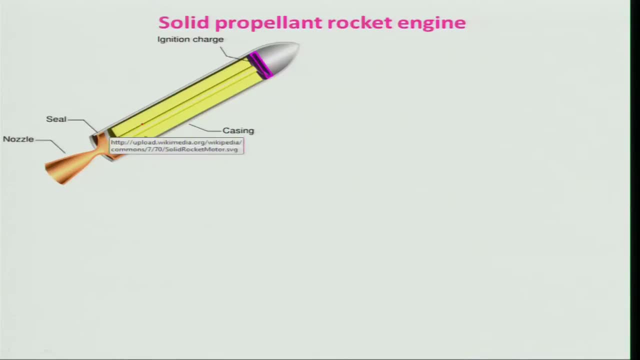 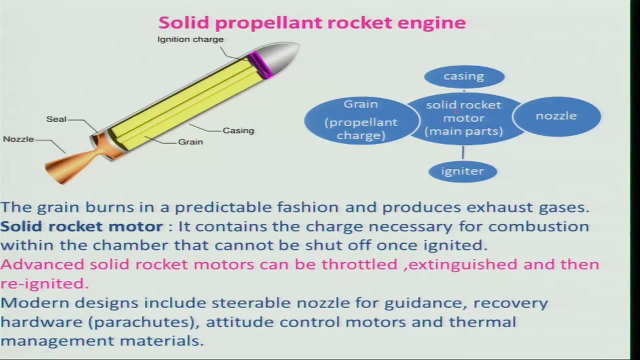 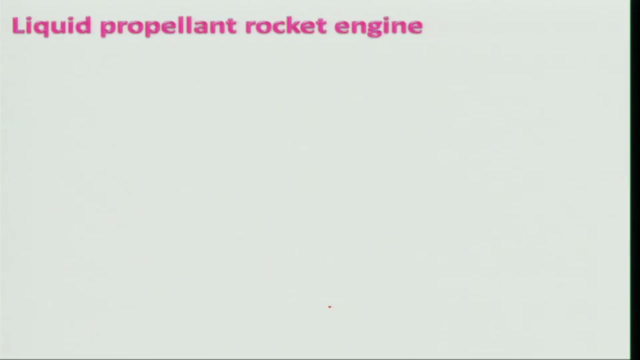 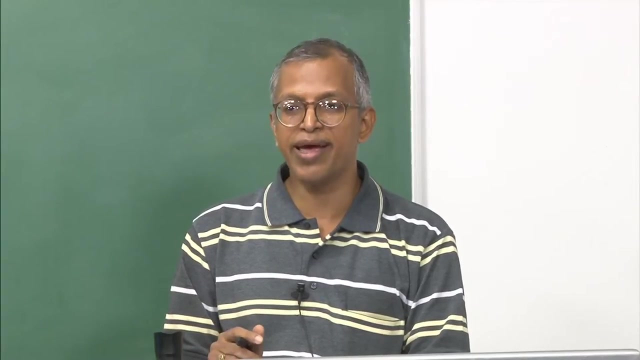 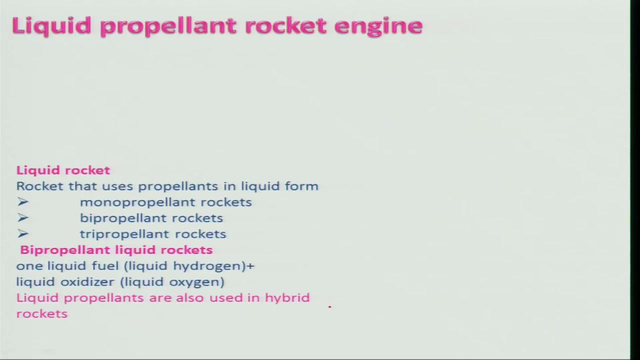 particularly in the aspect of the gas turbine and rocket engines. So let us look at solid propellant, rocket engines And Bipropellant, where you know like one is oxidizer, other is prop, other is a fuel, and try propellant which is really being used. But however, the three combination can be. 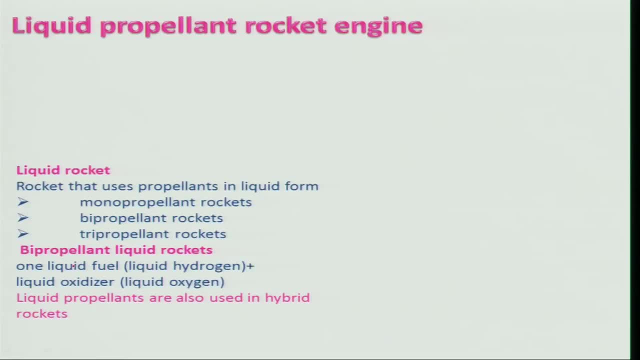 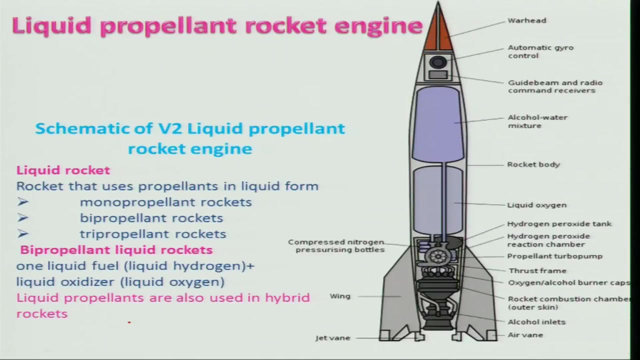 used. the example of Bipropellant is: the one is a liquid fuel, that is the liquid hydrogen, which is being used, and liquid oxidizer, like liquid oxygen, is being used as a propellant, And I will just show you a schematic signature. The second one is the liquid hydrogen: liquid hydrogen- liquid oxygen: one liquid liquid oxygen. 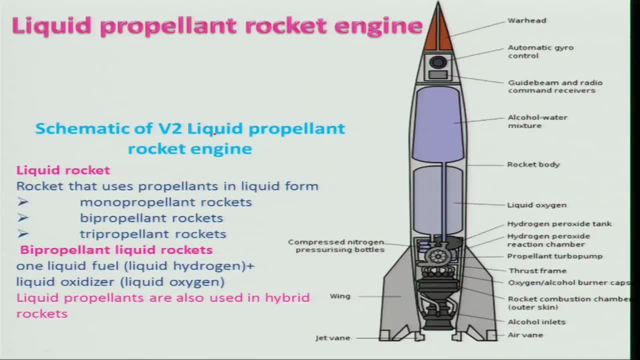 is being used. So liquid oxygen is used as a propellant, And I will just show you a schematic of the V 2 liquid propellant rocket engine which has created a havoc during the second world war, which was being what you call developed by Germans, And it was the first ballistic. 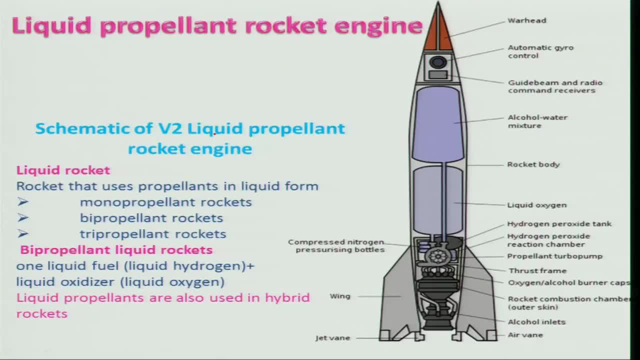 missile which was used in the entire world in 1942, kind of things, and it has, you know, like for producing this. 12000 people died just to produce this, several because of under the Nazi, whereas it has created lot of havoc in the England. 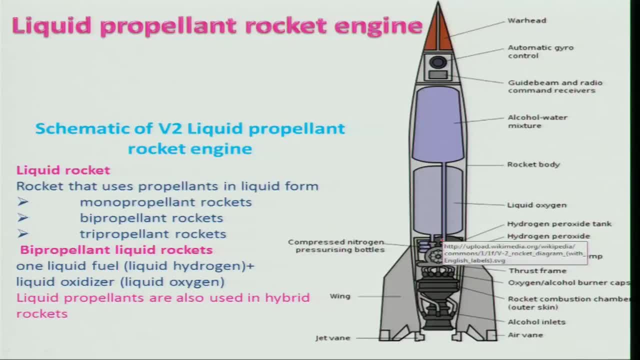 So this engine, if you look at shown here, which is having a war head, and this, of course, the gyro, is there automatic gyro guidance and control? it is based on the alcohol and water mixtures, right, And alcohol is nowadays not being used, of course, the liquid oxygen. 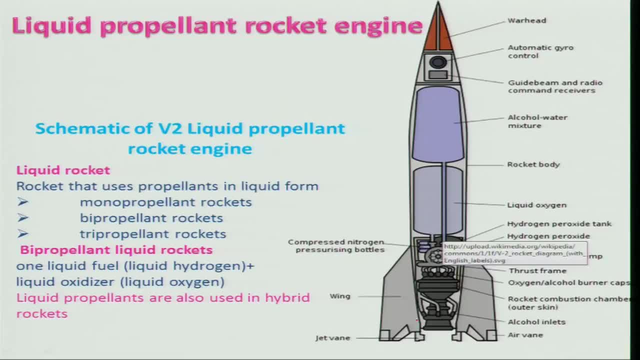 was being used. it is a quite compact engines and it produces thrust and it is having wing jet avance to control this engines. if look at your engine, is this much? I mean this is a very small compact. it is having a large amount of fuel and oxidizer, So also and 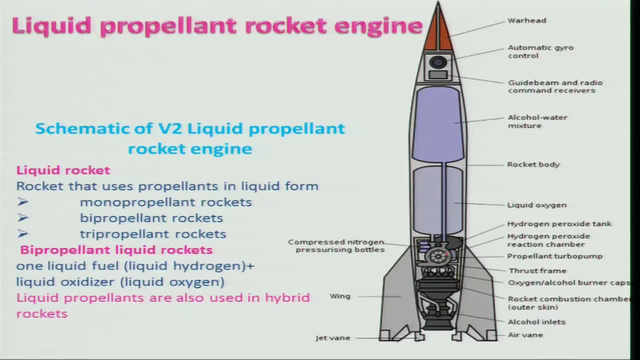 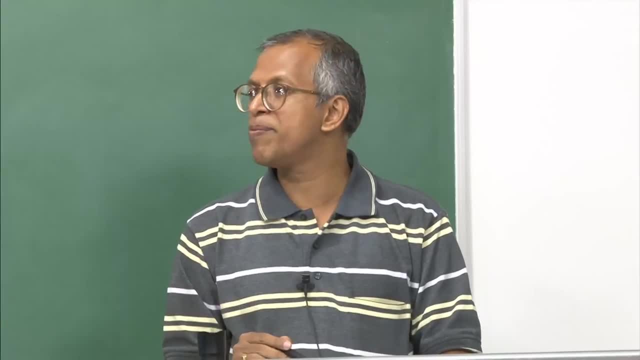 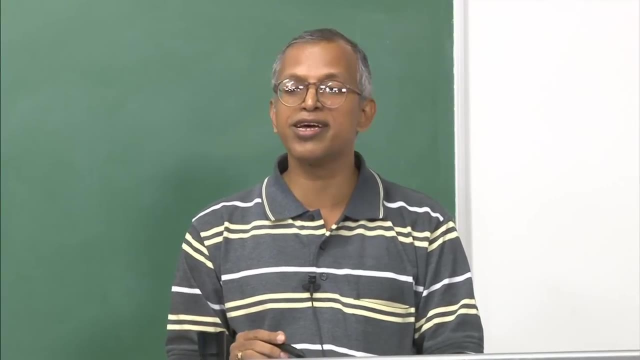 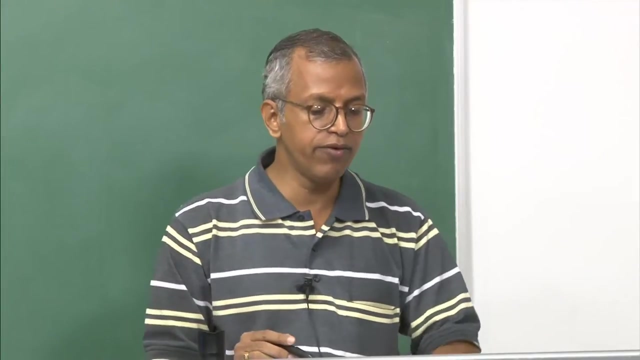 which is subsequently this V 2 rocket engine is being captured and taken to USA, England and Russia. they have further developed this engine. whatever engine we see, the father of those engines is basically V 2 rocket. So let us look at a hybrid engine where both the solid fuel, like grain, is being used. 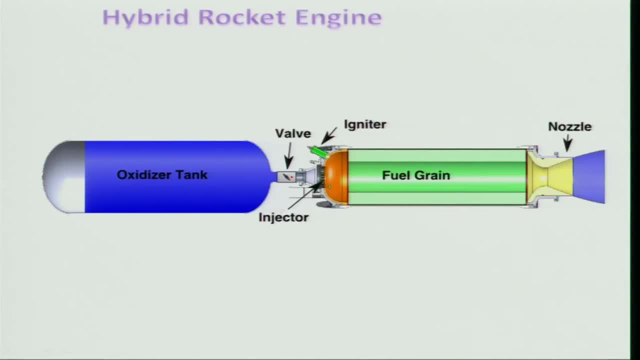 and oxidizer and it is having use because it is having several advantages over both the solid and the liquid propellant engines. So either one solid or even the gas or the liquid can be combined together. It is not the only the liquid and solid it can be combined and hybrid rocket engine.